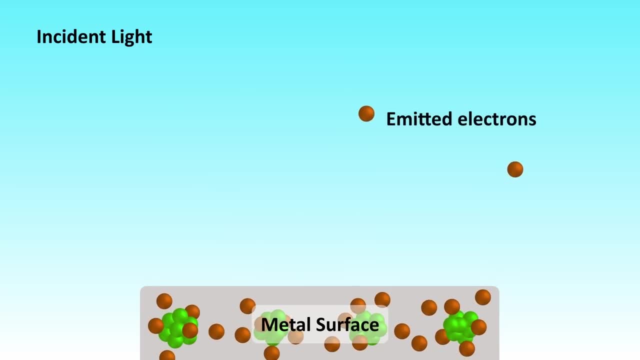 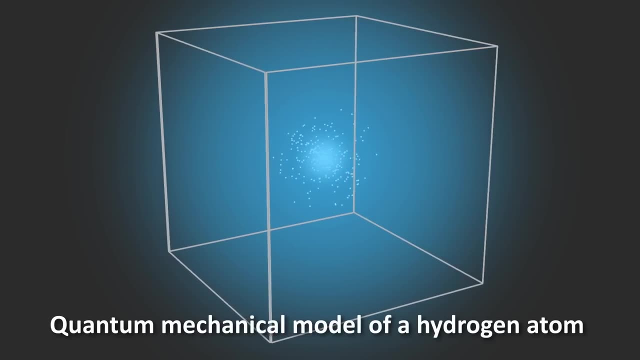 emitted from a metal plate only by light beyond a certain frequency, not intensity, And it helped advance the idea that quantum mechanics is the most accurate way to describe the true nature of reality. Fast forward some 120 years later to today and advancements in quantum mechanics. 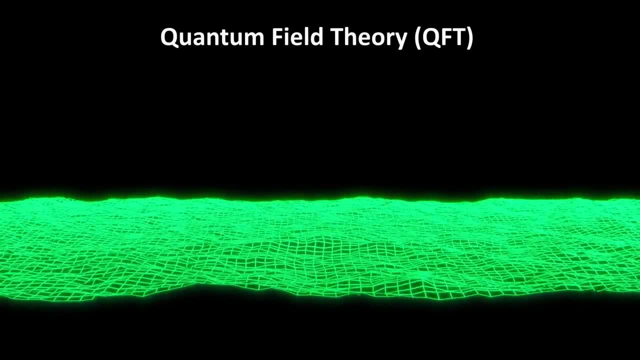 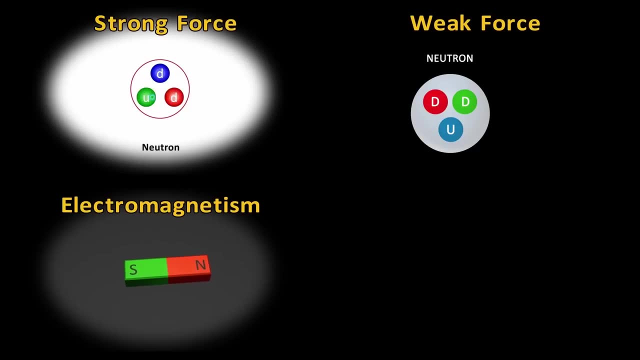 has led to a mathematical framework that brings us tantalizingly close to a theory of everything. This framework is called quantum mechanics, Quantum field theory. It's various aspects describing nearly all particles and forces in the universe. It's consolidated into the most accurate and proven theory of reality we have. 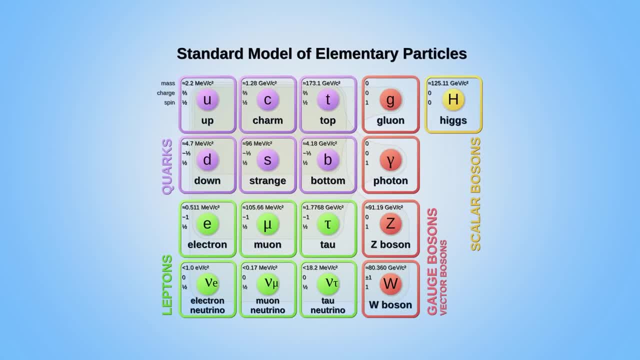 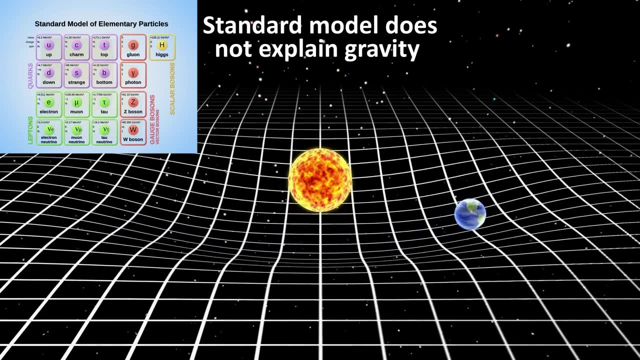 called the standard model. But we know this is not the final theory. It doesn't explain gravity. So we're still in search of that crazy new idea that could lead us to an even more accurate and complete description of the universe. Did I say crazy? Enter string theory Originally thought. 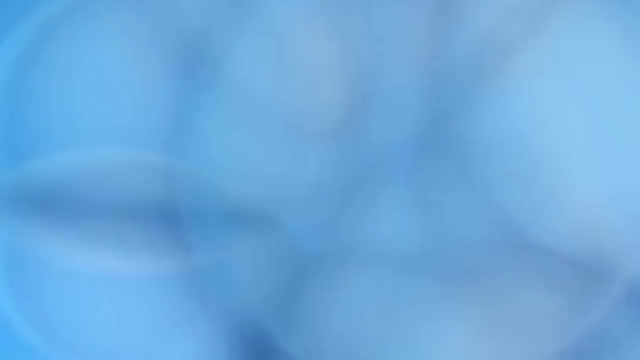 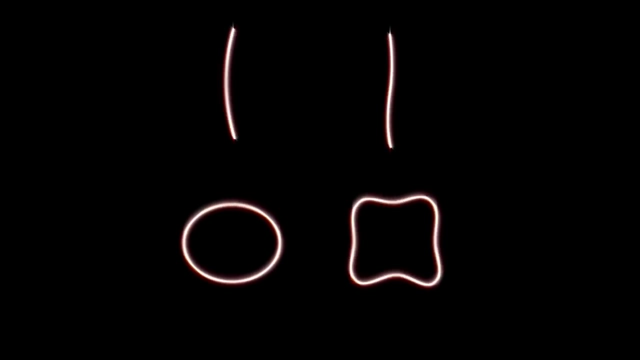 to explain hadrons, That is, particles like particles that are in the air, But they're not. They're like protons and neutrons in the late 1960s. This theory may seem insane, as it proposes crazy ideas such as a universe made of vibrating strings and with at least 10 dimensions, Mind you. 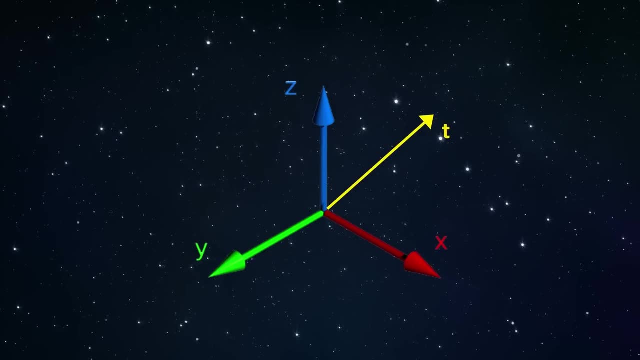 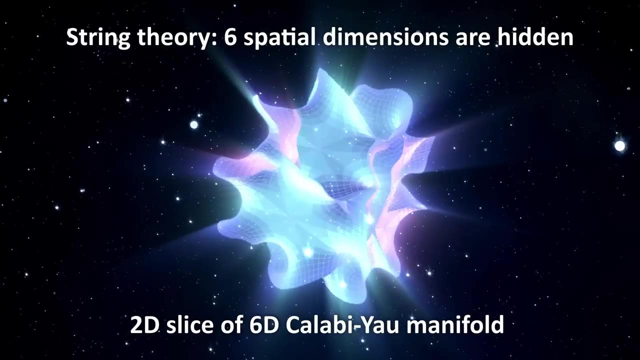 we only know of four: The three spatial dimensions and time. String theory claims that somehow at least six other dimensions have managed to stay hidden from even the best experiments we've made. But it appears to have an answer explaining gravity, And many physicists have spent nearly 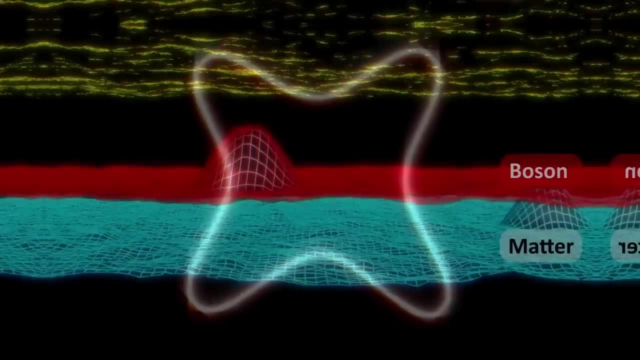 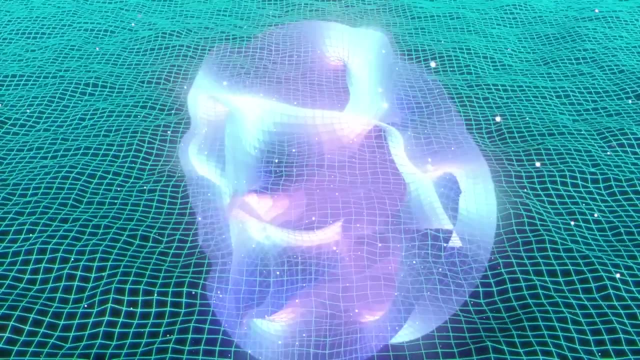 their careers studying it. The big question is: how do the crazy ideas of string theory fit with the now well-established quantum field theory and the standard model? Are they at all compatible? How are they different? Can they both be correct? That's coming up right now. 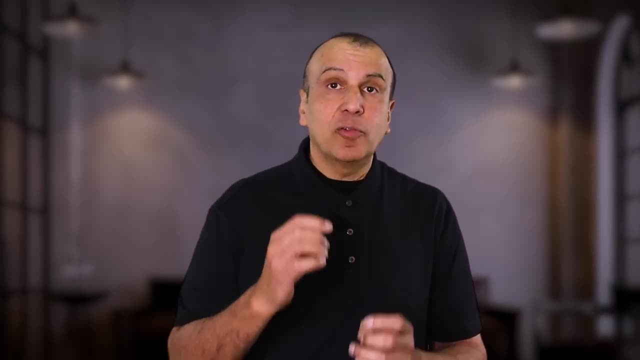 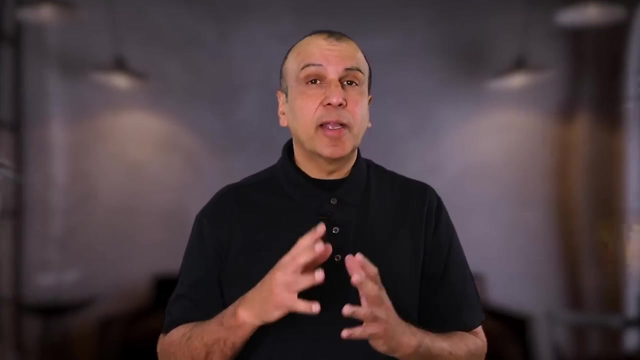 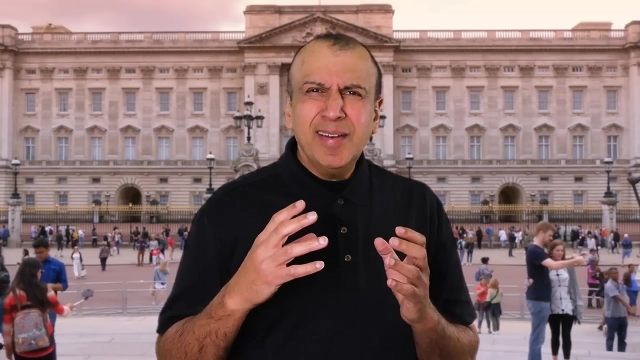 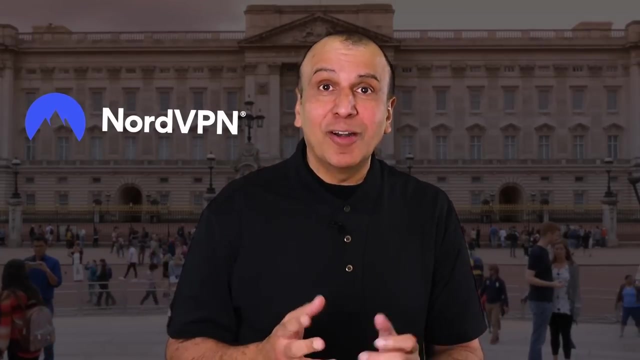 String theory and quantum field theory are both ways to model the universe in a…. Wait, is this Germany? Let's try that again. String theory and quantum field theory are both… In London. Oh, I get it now. It's because I'm using NordVPN, today's sponsor. 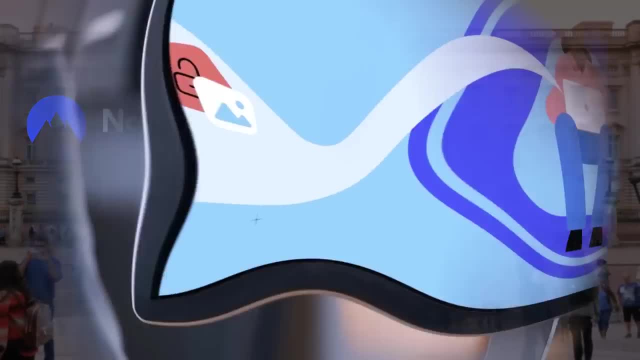 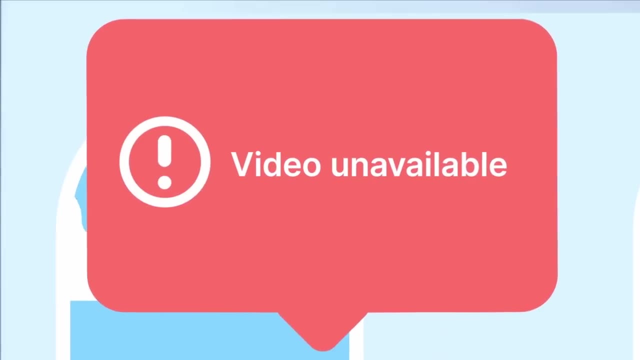 They can establish a secure encrypted connection between your device and a remote private server in one of 50 plus countries like Germany or the UK. Your virtual location can be in any of these countries. So, for example, if you're currently geo-restricted from certain online. 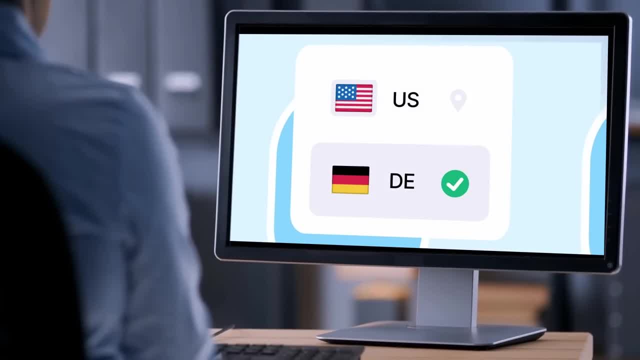 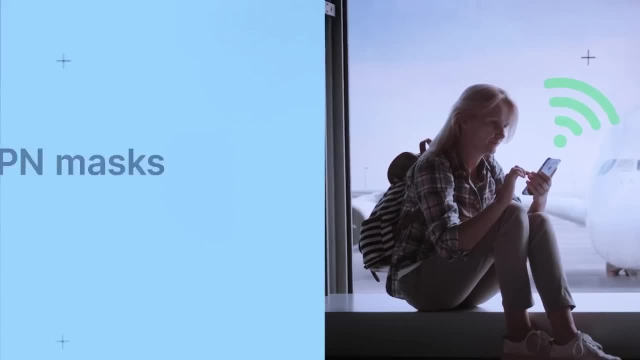 content. it's not a problem with NordVPN. In addition, it encrypts all your data, so third parties like your Snoopy service provider can't know your online activities And your data is secure from hackers. They have a special offer for Arvin Ash viewers right now. 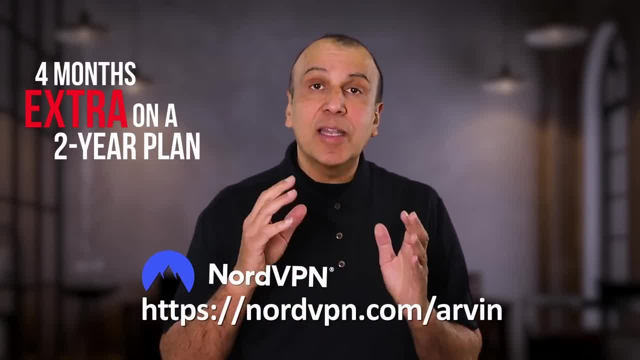 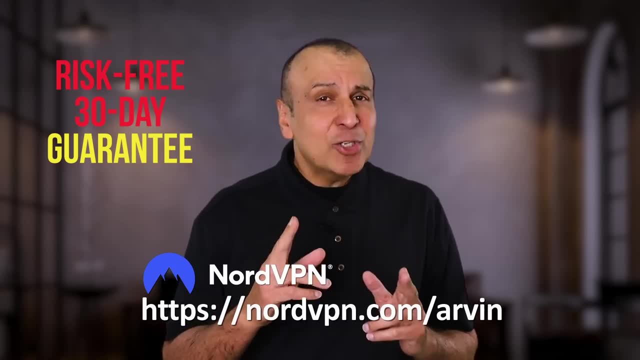 You can get 4 months extra on a 2-year plan if you click the link in the description. NordVPN slash Arvin And it's completely risk-free with a 30-day money-back guarantee. Give it a try and stay safe online Now. where were we? 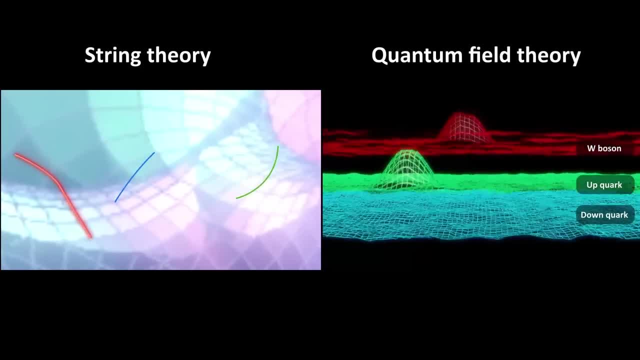 String theory and quantum field theory are both ways to model the universe in a…. String theory and quantum field theory are both ways to model the universe in a…. String theory and quantum field theory are both ways to model the universe in a useful mathematical framework, but they approach the fundamental nature of the universe from. 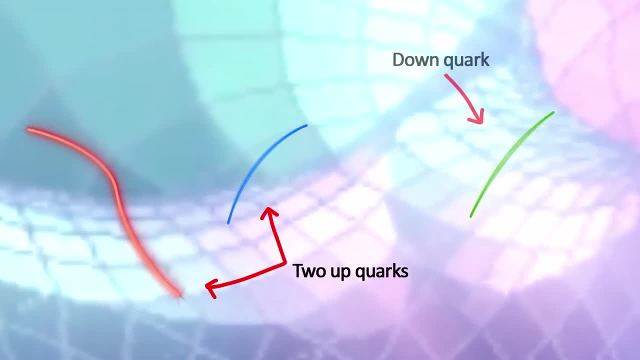 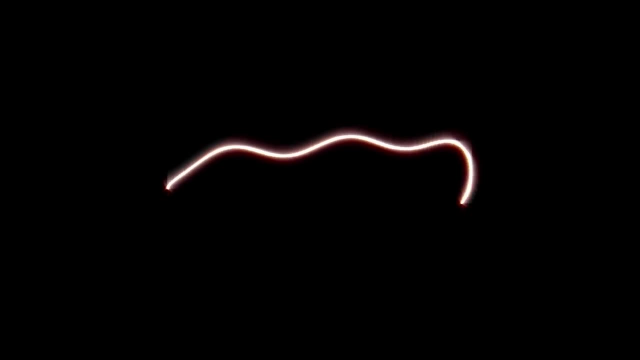 different perspectives. String theory is a theoretical framework that posits that the smallest building blocks of the universe are not zero-dimensional, point-like particles, but tiny one-dimensional strings that vibrate at various frequencies and in different dimensions, and that different combinations of frequency and dimensions can describe. 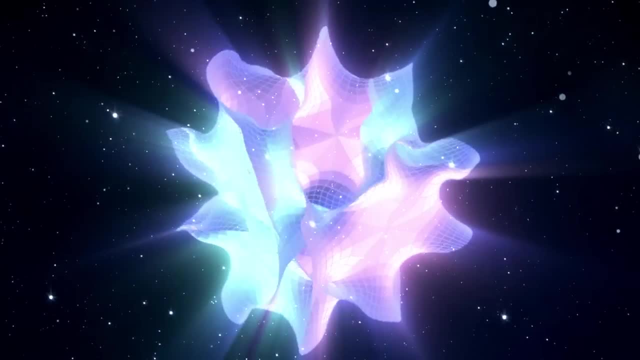 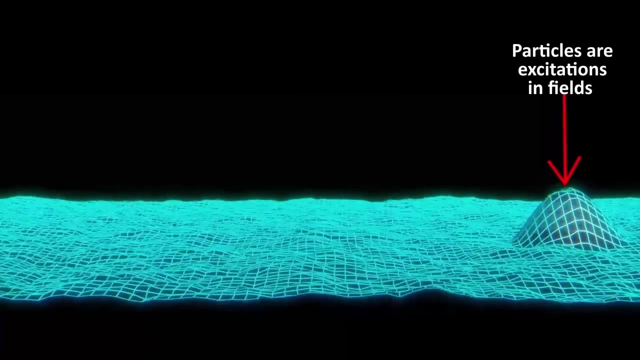 all the different types of matter, forces and energy in the universe. On the other hand, quantum field theory postulates that all particles are excitations in fields that span the entire universe and that forces are due to the interaction of these particles. 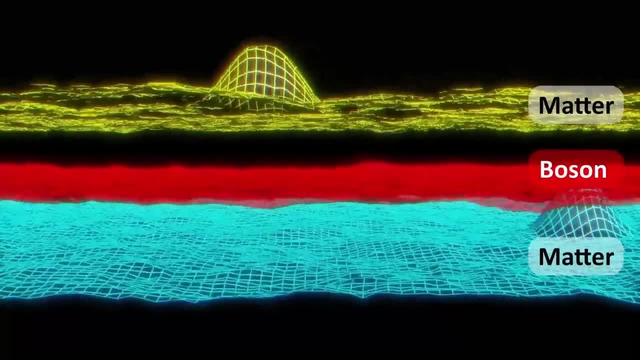 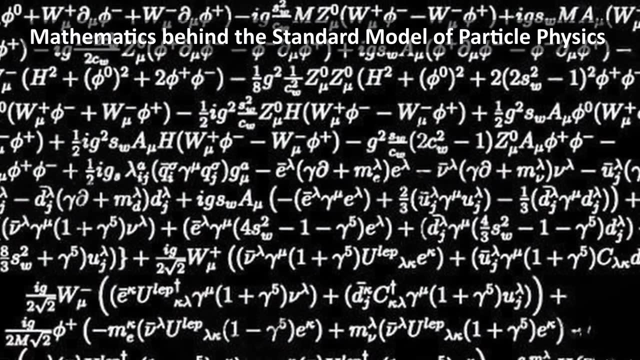 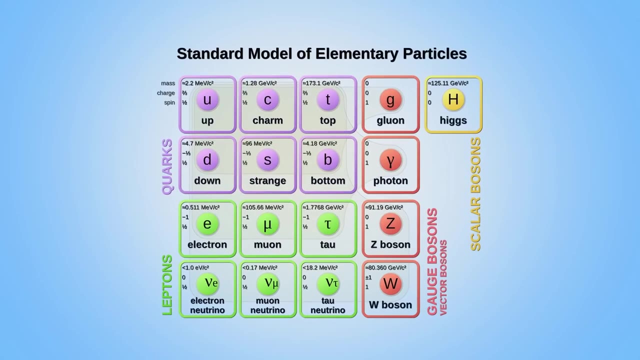 mediated by other particles called bosons. It is the mathematical framework describing how particles and forces interact at the subatomic level, And our best and most accurate understanding of the universe based on this framework is consolidated in what is known as the standard model of particle physics. This standard model is represented by 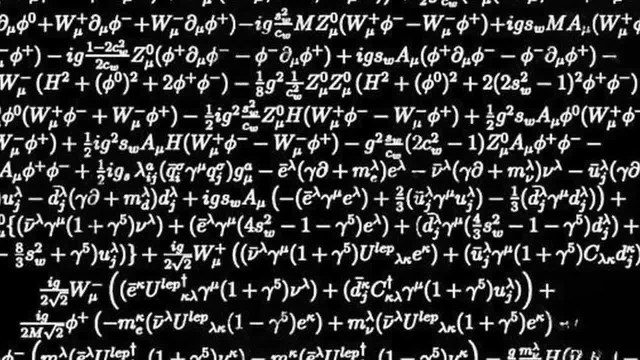 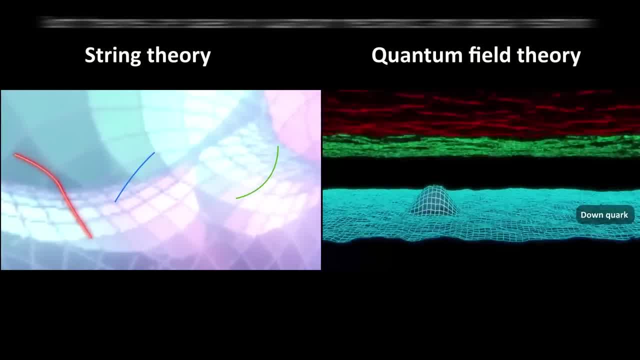 all the equations you see here. If you want to know more about what these equations mean, I have a dedicated video here on that. Both string theory and quantum field theory are based on the principles of quantum mechanics and special relativity And, just like quantum field theory, is a mathematical framework. 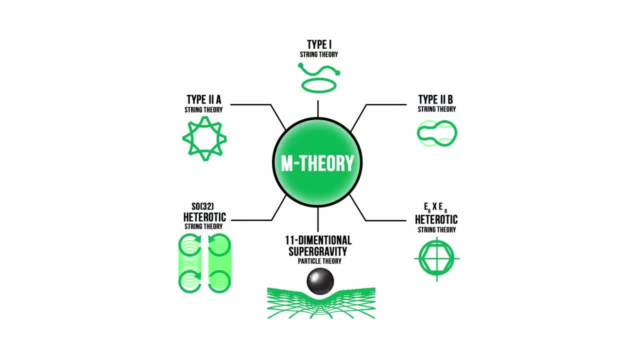 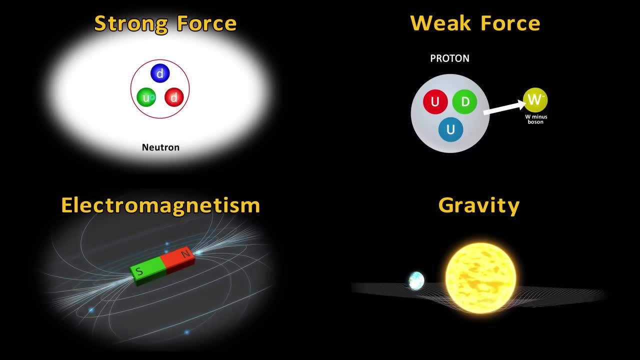 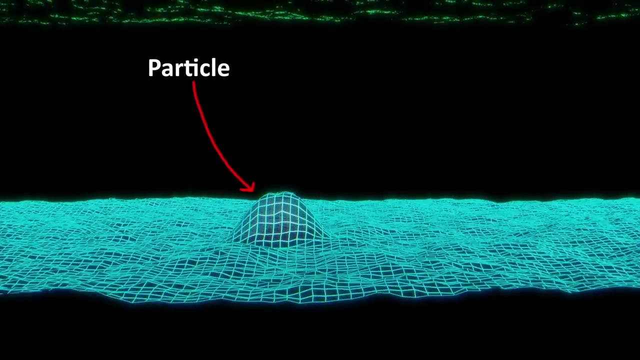 so is string theory. There are several string theories, all related to a deeper overarching theory called M-theory. Both theories, in principle, can mathematically describe all particles and forces. But we know quantum field theory or Q of T works. In fact it is the most accurate. 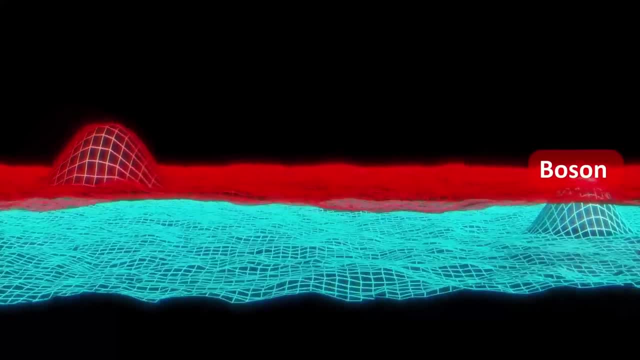 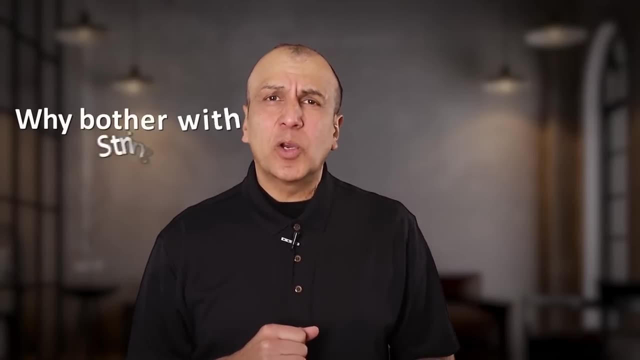 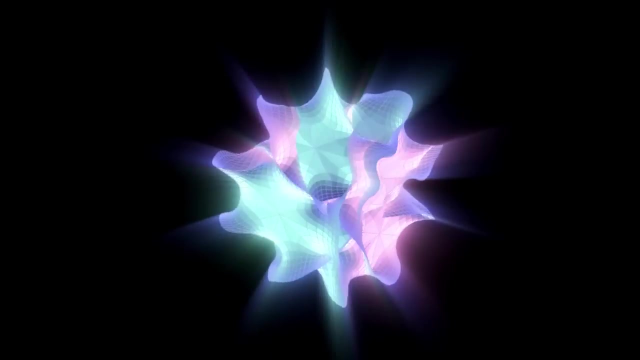 theory we have ever had. Its predictions concur with experimental results, in some cases to 10 parts in a billion. So why do we even bother with the crazy ideas of string theory? The biggest reason is that it so happens that a certain combination of a closed string vibrating 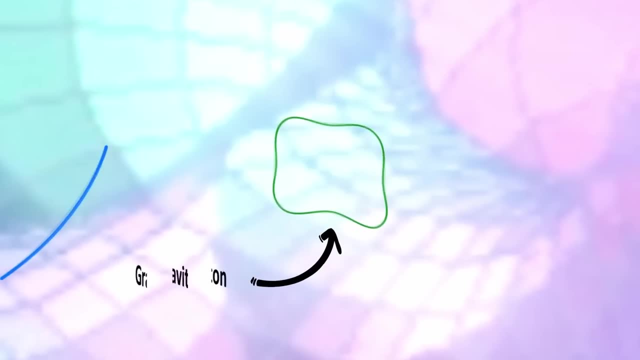 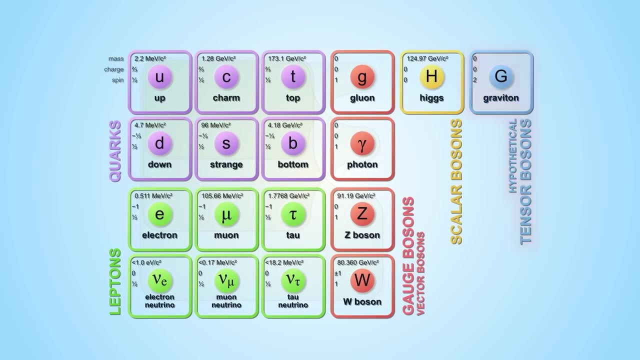 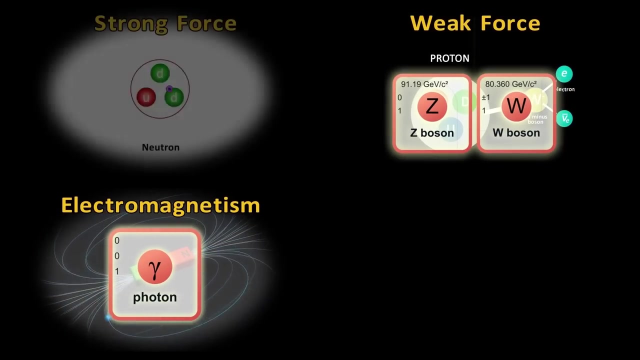 in the center of a particle is called a gravitational force or a gravitational force. The gravitational force is the theorized missing boson particle of the standard model that would carry the gravitational force, similar to the way photons carry the electromagnetic force, W and Z bosons carry the weak force and gluons carry the strong force. 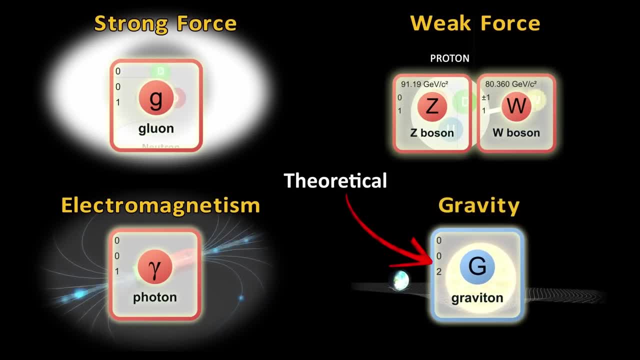 Keep in mind that gravitons are theoretical only. They have never been detected. They are predicted by string theory, and that is why the theory was so popular some decades ago. Physicists thought that it could provide the mathematical leap we needed to integrate gravity. 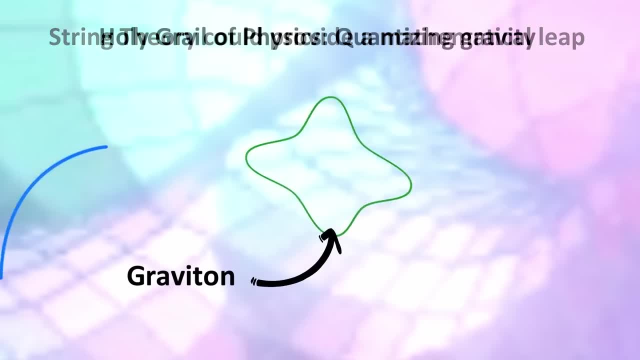 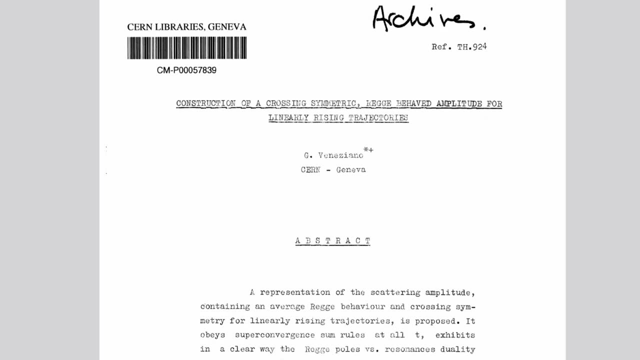 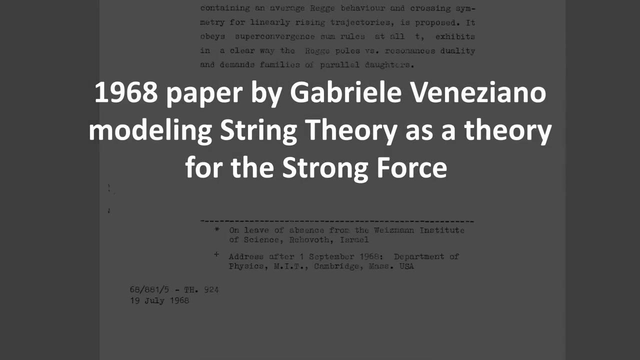 into quantum field theory, And if that could be done it would solve the holy grail of physics, the quantization of gravity. Interestingly, string theory was first proposed in the late 1960s and early 70s to describe the forces that keep hadrons like protons and neutrons. 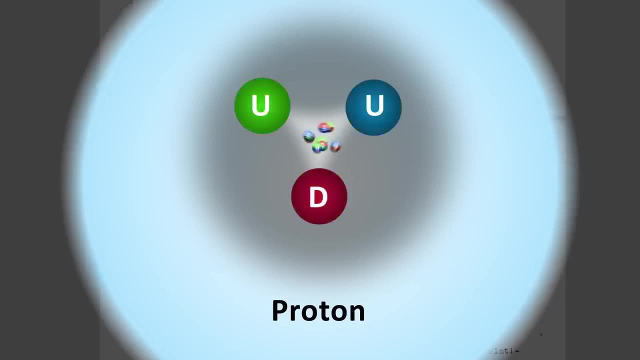 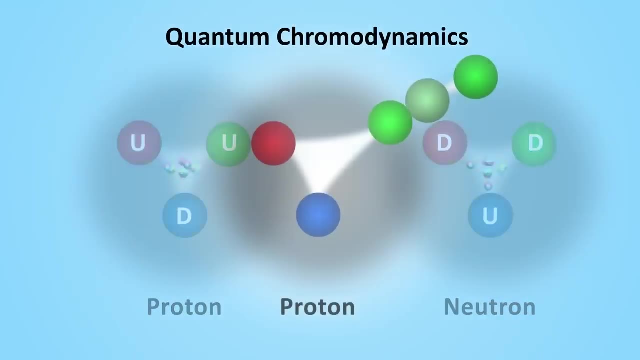 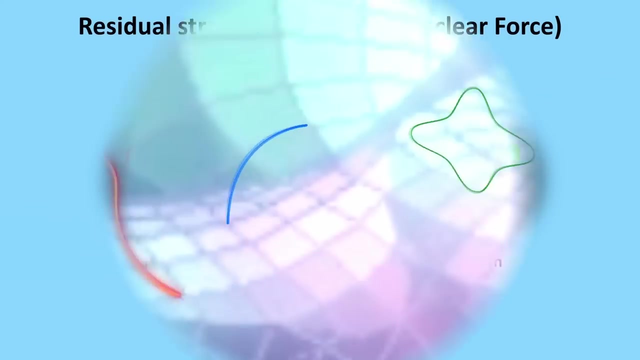 glued inside the nucleus of atoms, But it turned out that it was not needed, because a quantum field theory called quantum chromodynamics, QCD, worked quite well And it is today the established theory that quite accurately describes the strong nuclear force. However, this exercise with string theory was not a complete waste, because it led to scientists. 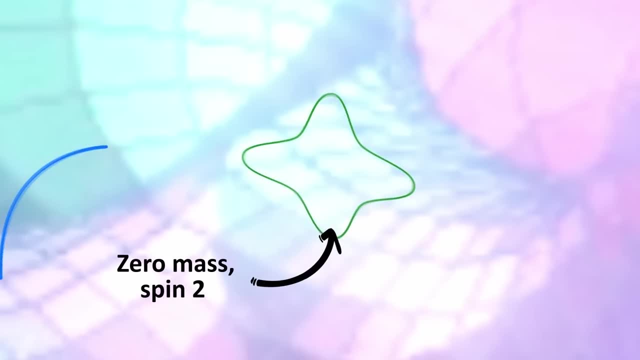 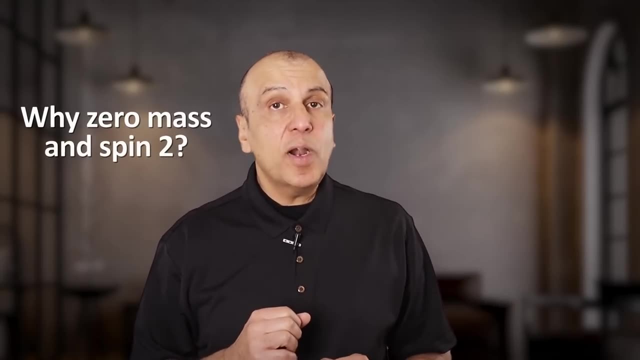 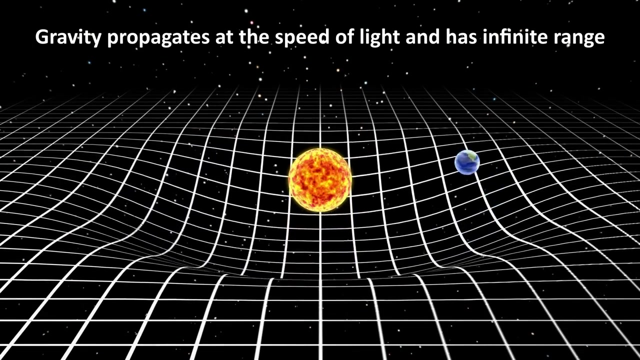 finding that you could mathematically model a particle with zero mass and spin of 2.. These are the properties of a graviton. Why is zero mass and spin of 2 required to model a graviton? Well, there are two main reasons for this. One is that gravity propagates at the speed of light and has 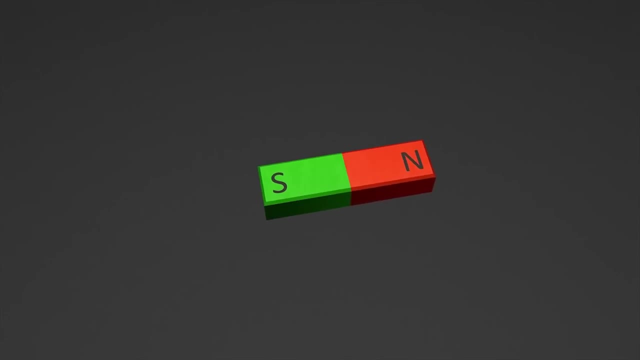 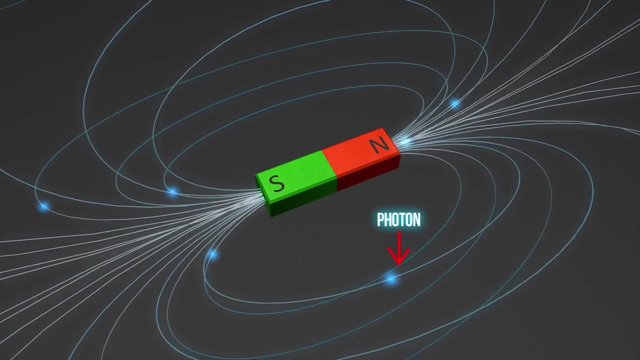 an infinite range. Only a massless boson particle could have such properties. It is akin to electromagnetism, which also obviously propagates at the speed of light and has infinite range, And its carrier particle is the massless photon. The spin of 2 requirement is a bit complicated. 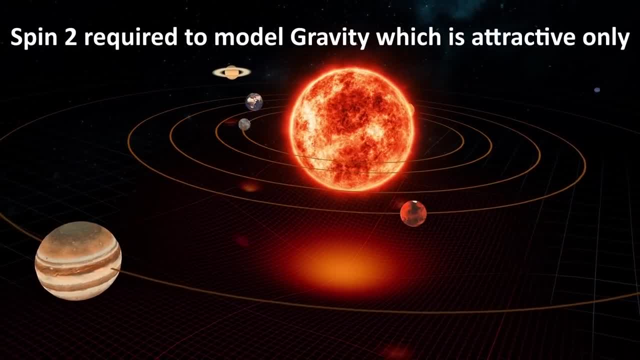 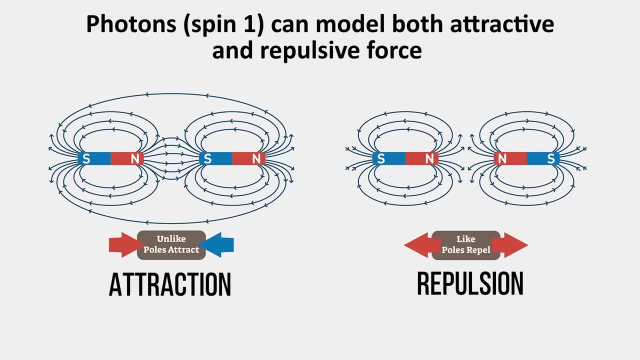 to understand. There are two main reasons. First, spin of 2 is required to model an exclusively attractive force, which is what gravity is. Spin of 1,, for example, like in photons, the carrier's of electromagnetism can model both a repulsive and attractive force. Second, a graviton must. 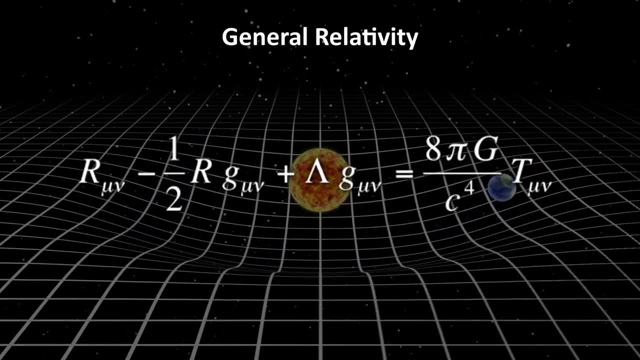 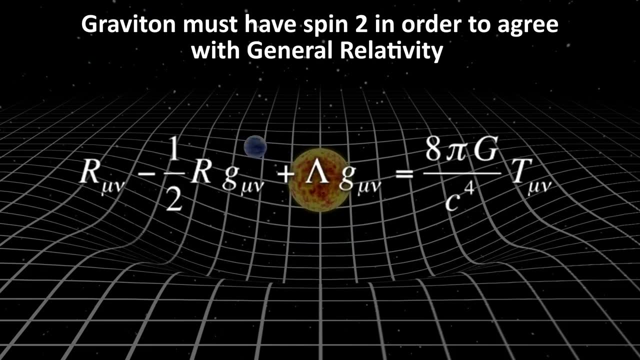 have a spin of 2, because that's the way spacetime would have to be quantized in order to agree with general relativity, which we know works and is the current best model we have for gravity. So whatever theory we get has to agree with general relativity. 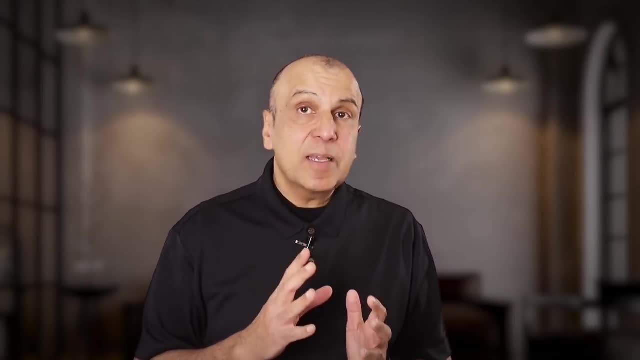 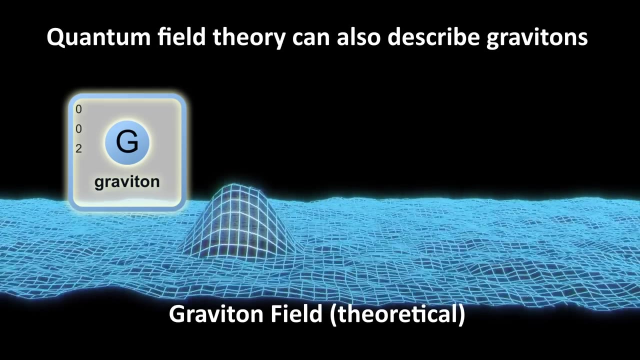 But simply having a description of gravity in string theory is not something to get too excited about, because quantum field theory can also describe gravitons as excitations in a reticle graviton field. But the problem with trying to quantize gravity in quantum field theory 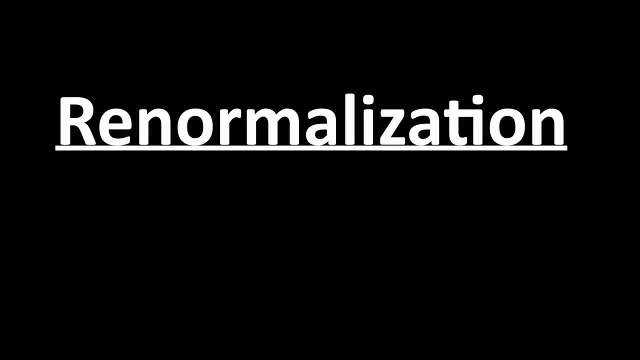 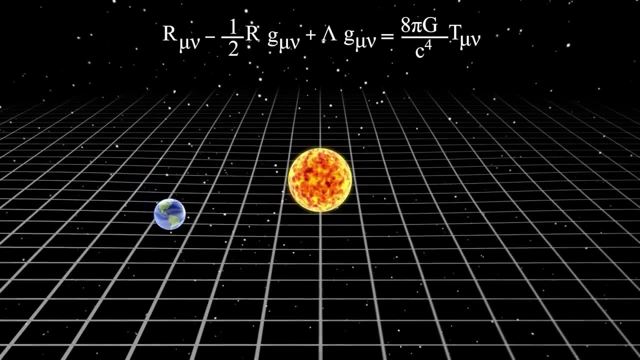 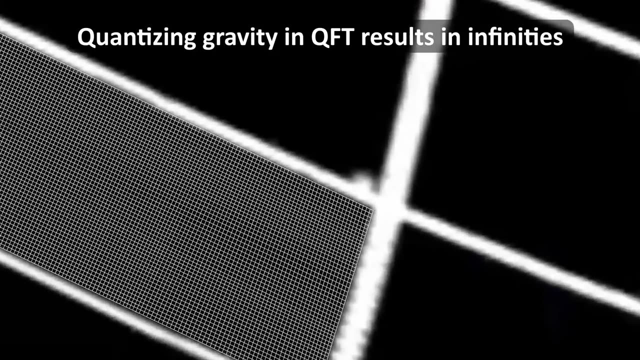 is something called renormalization. This is the procedure of making a theory valid to infinitesimally small lengths. When we try to do this, that is, when we try to mathematically quantize spacetime itself, instead of keeping it as a background on which fields exist, we get infinities in the 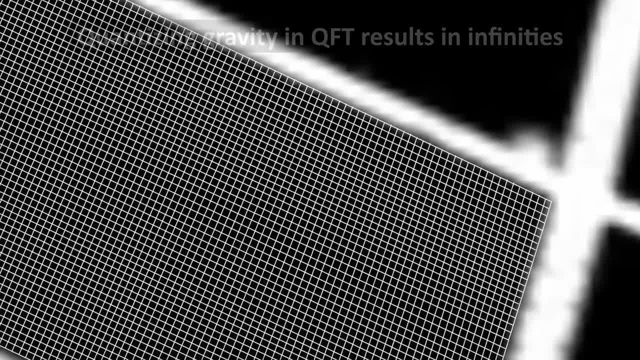 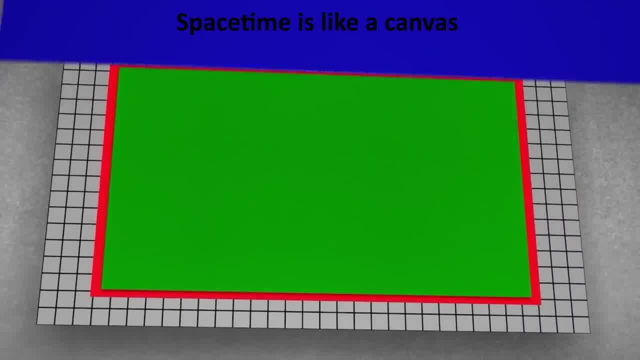 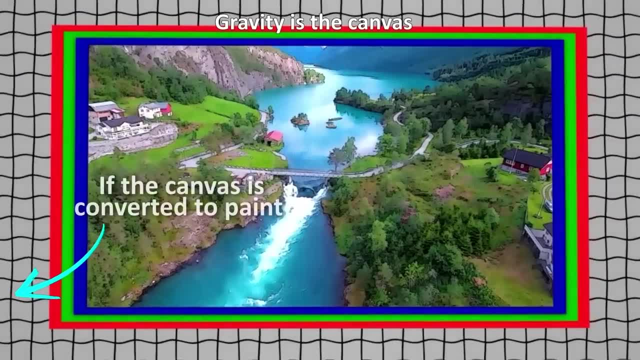 equations, So quantizing gravity using QFT doesn't really work. The analogy can be made something like this: Spacetime is the background on which quantum fields exist, like paint exists on a canvas. So when you try to make the canvas itself into a paint, 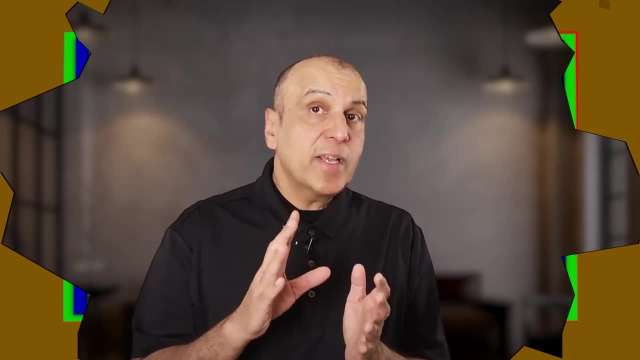 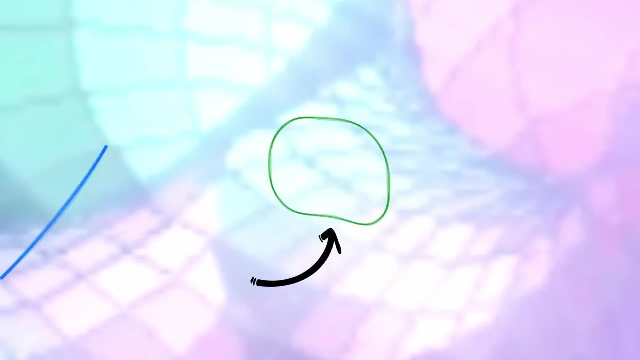 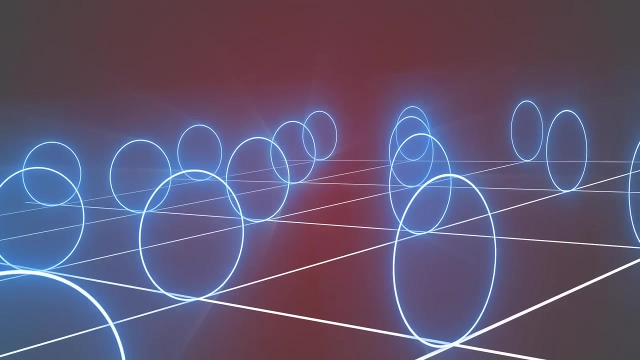 the painting falls apart. If you want to know the details of what exactly falls apart, I made a video about it right up here. Unlike QFT, string theory solves the issue of quantizing gravity, But there's a big price we pay for being able to do so, And that is we have to contend with. 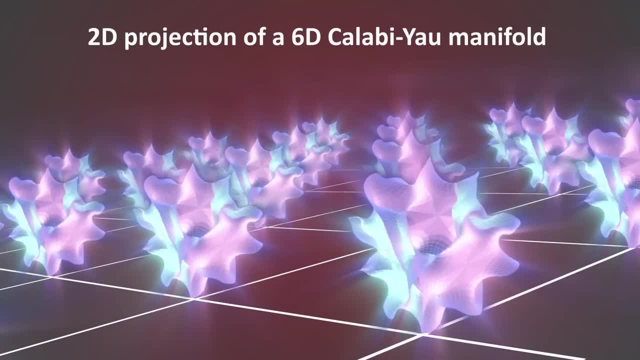 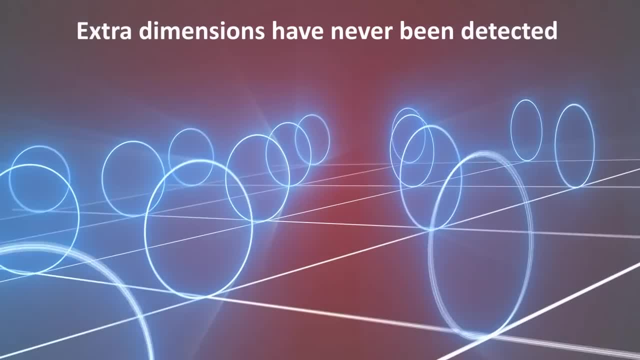 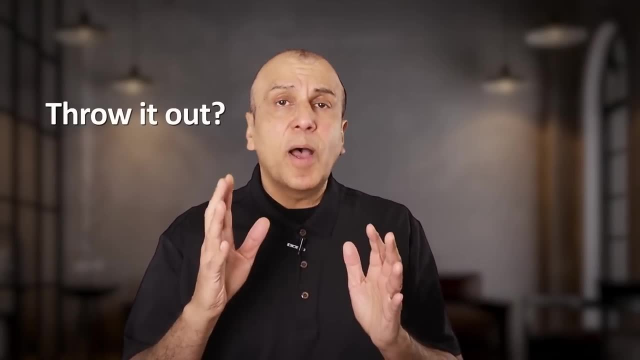 trying. Scientists have conducted test after test to try to detect these extra dimensions, but they've all failed. Now you might say, well, we need to throw it out then and come up with some other crazy idea. But not being able to find these extra dimensions does. 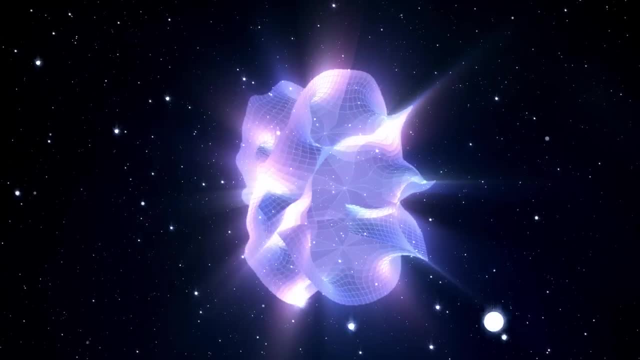 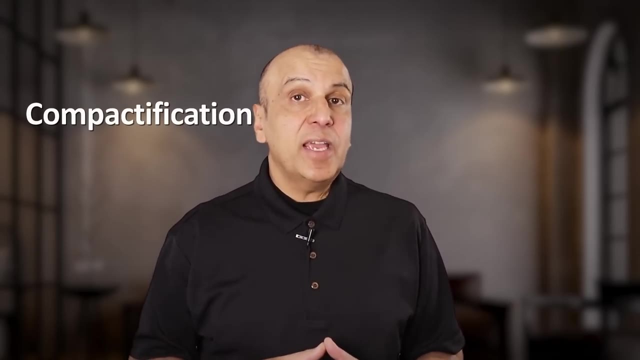 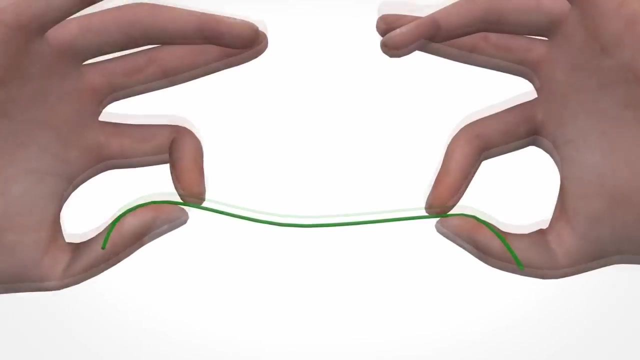 not necessarily make string theory incorrect. Scientists have come up with explanations about where the missing dimensions might be. One is compactification. It can be thought of like this: Imagine holding a piece of thread or floss. From far away, it looks like a thin, one-dimensional. 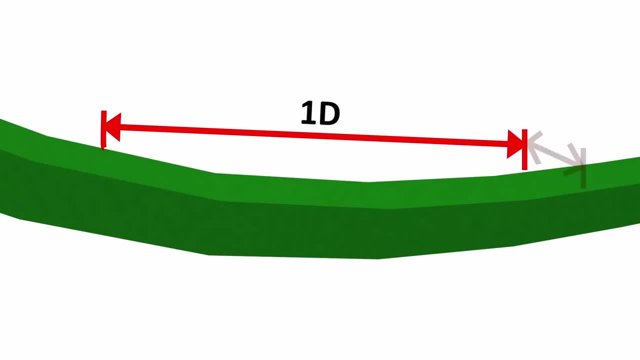 line. But as you look at it more closely you realize that it's not just a line. it has a two-dimensional surface And if you look at it under a microscope you would see that it has an intricate third-dimensional structure. The idea is the same for string theory. We just see objects from a point of view. 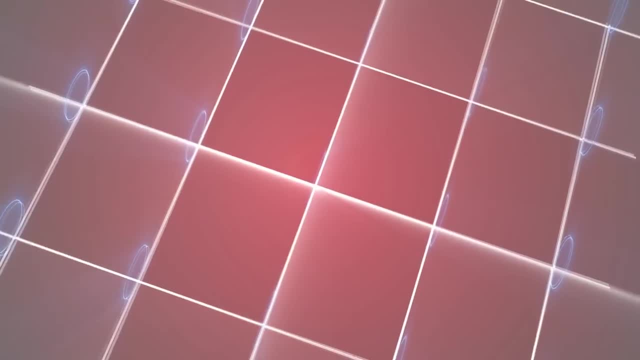 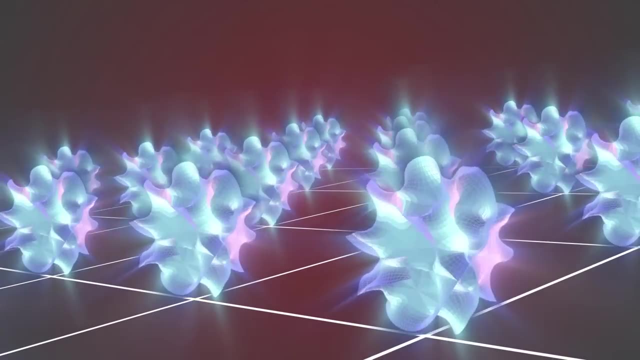 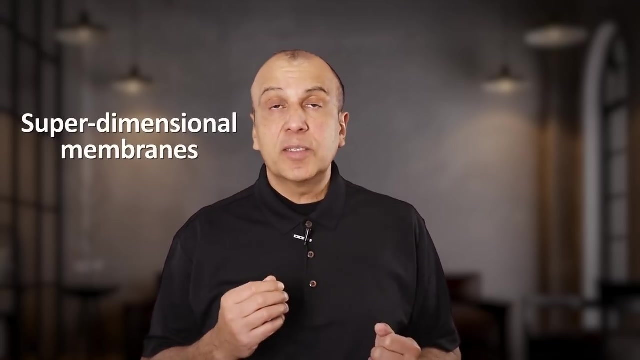 where things look three-dimensional. But if you could zoom in incredibly close, closer than we are technically capable of doing today, we would discover compacted dimensions that are hiding from us. Another possible solution to the missing dimensions is that there could be superdimensional brains or membranes. 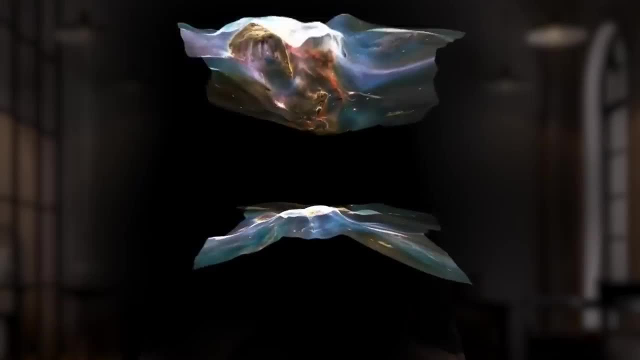 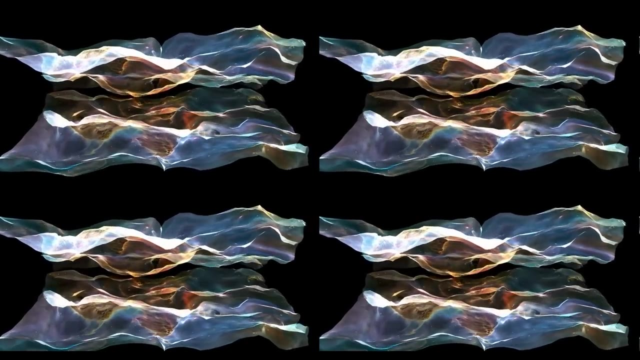 The idea here is that the universe may have more dimensions than we have access to, That there could be a fourth spatial dimension, And that these are isolated from other dimensions. We would have to exist outside of our local universe, And then we would have to leave it. So if we want space, we have to move it. But this is not the only way to go. You have to move it. You can go out and explore it. You will find something there. You can see it there, You will find it. 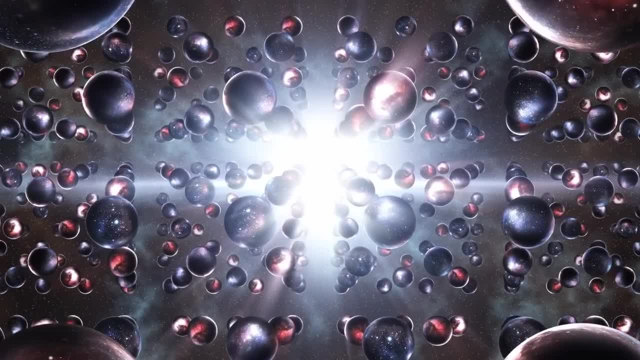 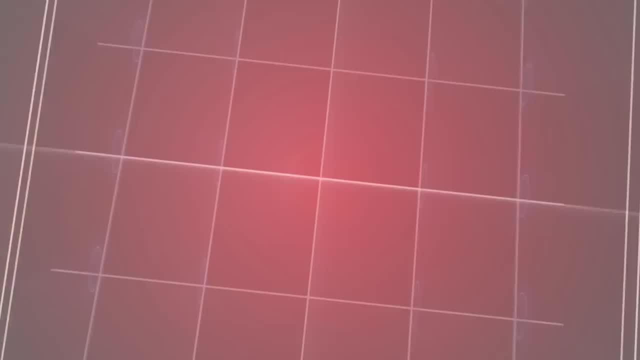 You will find it. You will find something here, You will find something there of our local brain to see these extra dimensions. The problem is that detecting dimensions on such tiny scales requires such large energy levels that, in practice, we can't verify it with our 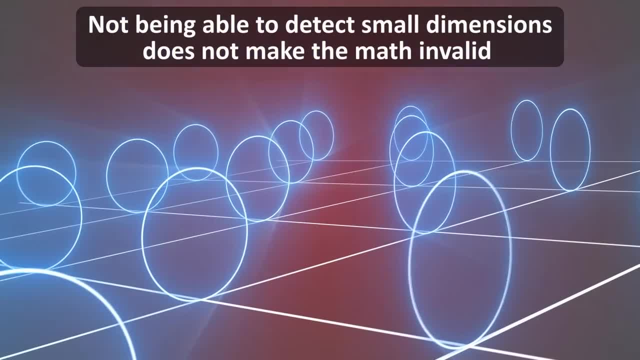 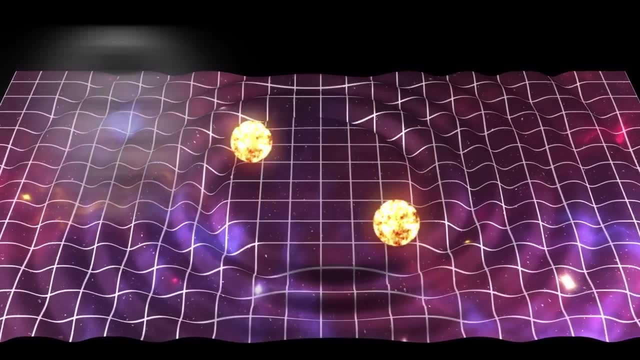 current technology, But this doesn't mean that the mathematics of higher dimensional spaces is invalid. After all, it took 100 years to detect gravitational waves, which were predicted by Einstein way back in 1916 and not discovered until 2015.. Maybe we can still work with string. 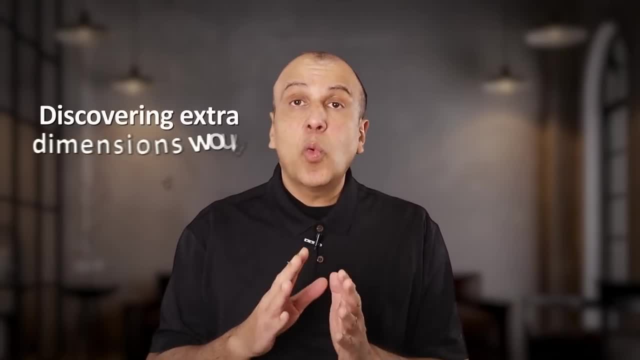 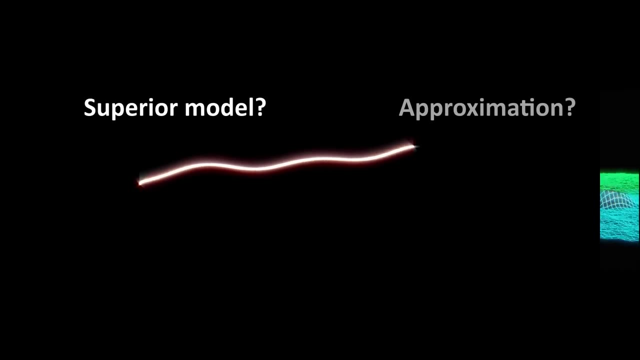 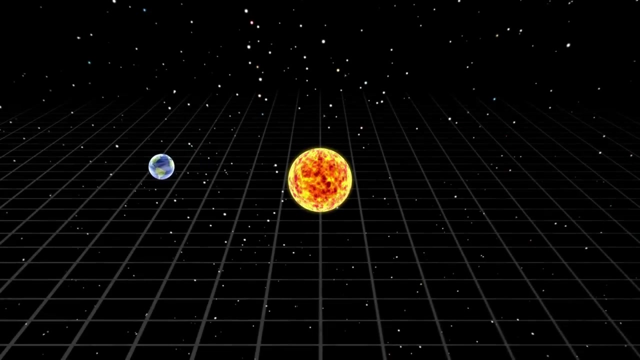 theory. If we could detect these extra dimensions, the reward would be staggering. It would be significant evidence indicating that string theory is likely the superior model of the universe and that QFT is simply an approximation. This would be similar to the way we found how general relativity 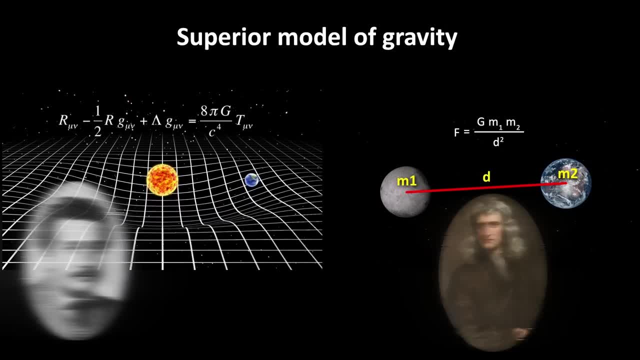 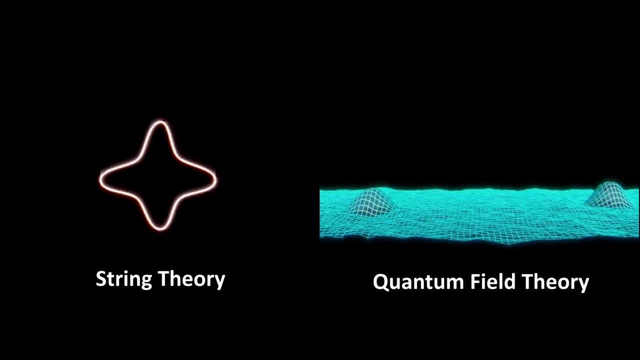 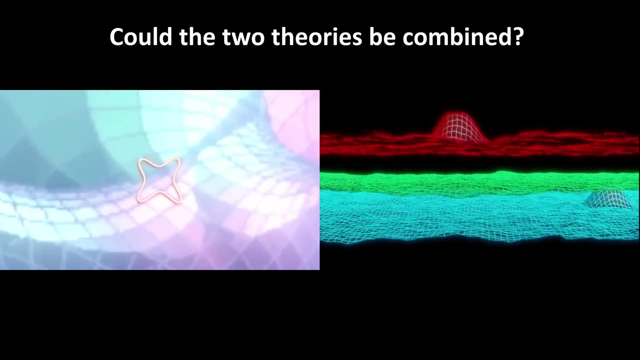 is a superior model of gravity to Newton's and that Newton's equations are just a good approximation. Could the two theories, quantum field theory and string theory, be combined To make a kind of composite theory? It doesn't seem so. The main problem is the extra dimensions. 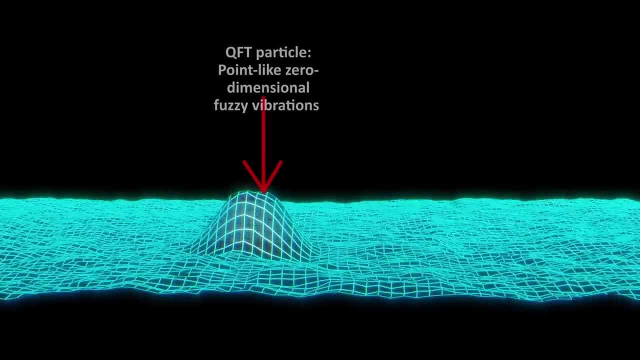 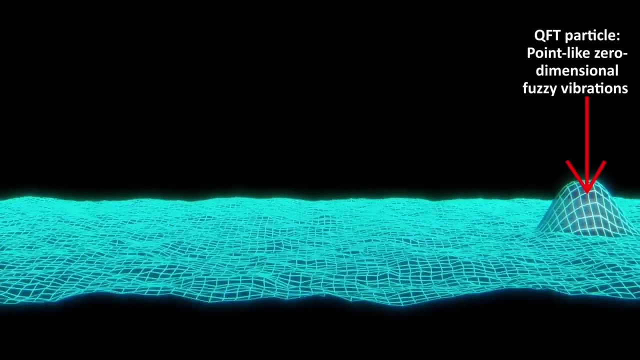 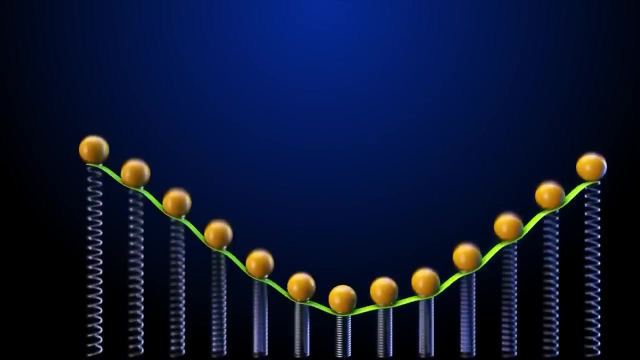 but are there any similarities? In QFT we define particles as point-like fuzzy vibrations having zero dimensions. They have no defined size. They are excitations in a field that exist in four dimensions: three spatial and one time, As I showed in a prior video. 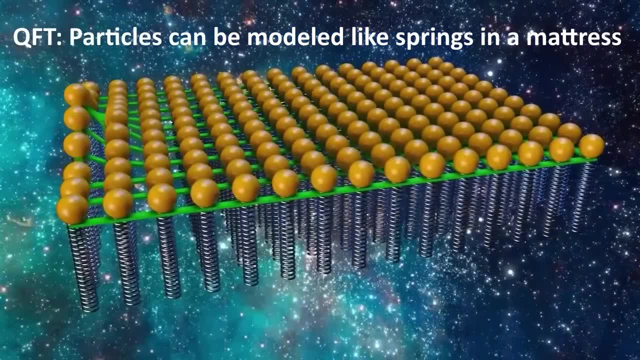 they can be mathematically modeled like oscillating springs in a mattress. So what is a string theory? Well, string theory is a kind of composite theory. The mattress can be thought of as the field, So the universe could be looked at as a bunch of 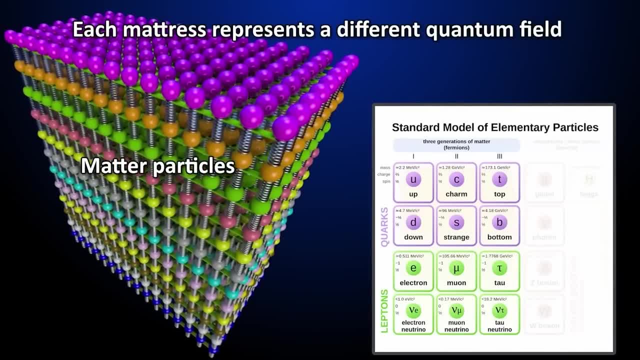 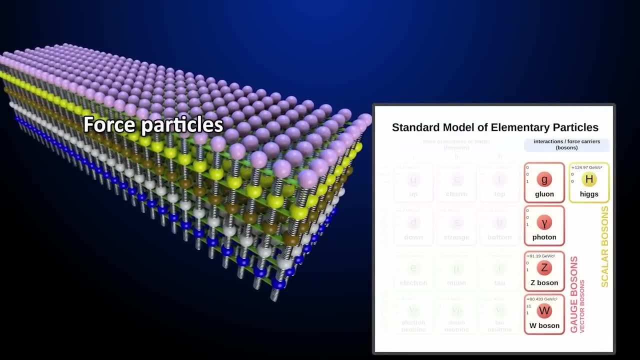 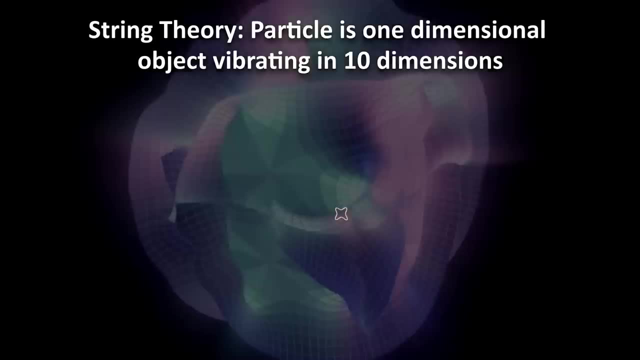 mattresses with springs oscillating. The different energy levels of the oscillations would correspond to the number of particles. In other words, the amplitude of the excitation represents the number of particles. In string theory, a particle is a one-dimensional object vibrating in at least 10. 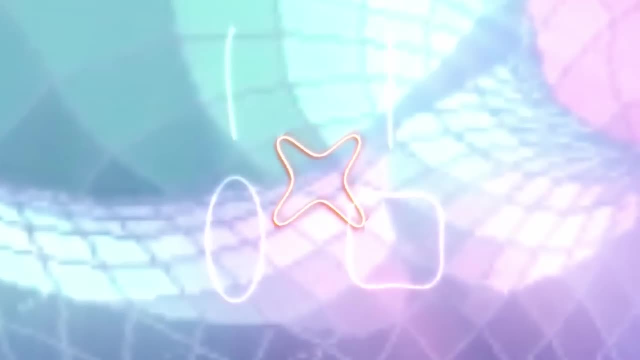 dimensions. It has a length, but no width or height. It can be an open or closed string, similar to a rubber band. It can be an open or closed string, similar to a rubber band. It can be an open or closed string, similar to a rubber band. 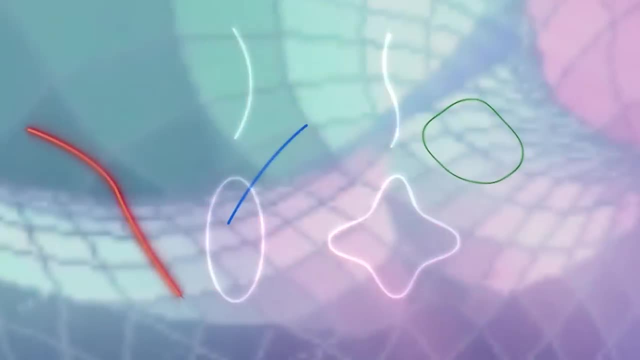 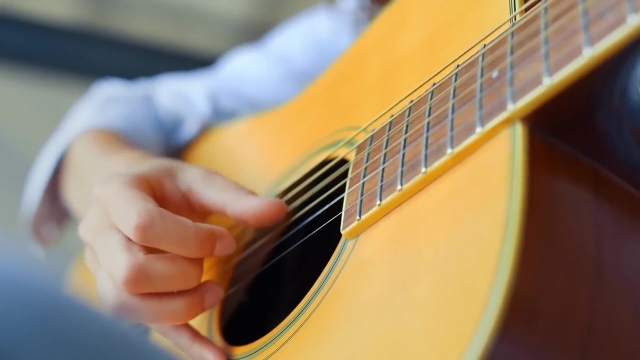 This 1D string can have a size. It's near the Planck scale, That's about 10 to the negative 33 centimeters. You can think of this as analogous to the strings in a guitar. It can vibrate to make sounds and just like the frequency of the vibration determines the pitch of the sound, 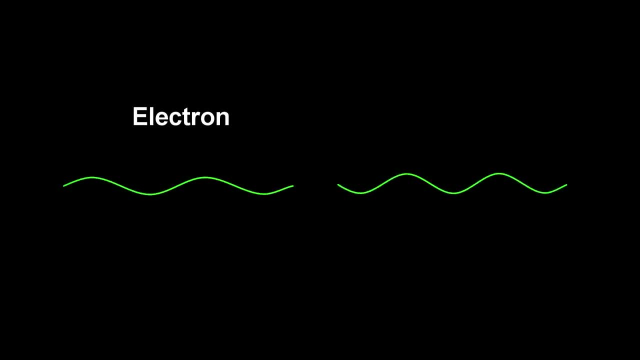 the frequency of strings in string theory determines the type of particle it is. So one string can act like different particles depending on how it vibrates and in which dimension it vibrates, But similar to how the amplitude in QFT corresponds to the number of particles, the amplitude of the vibrations in string theory. 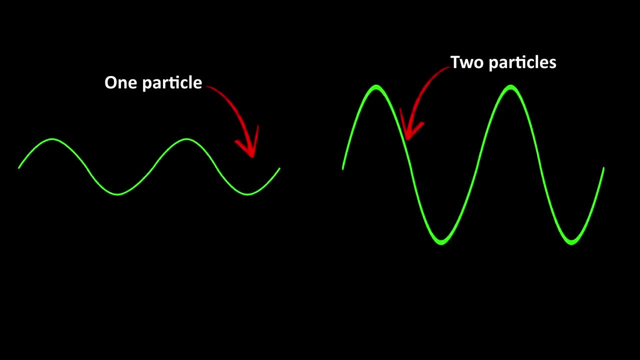 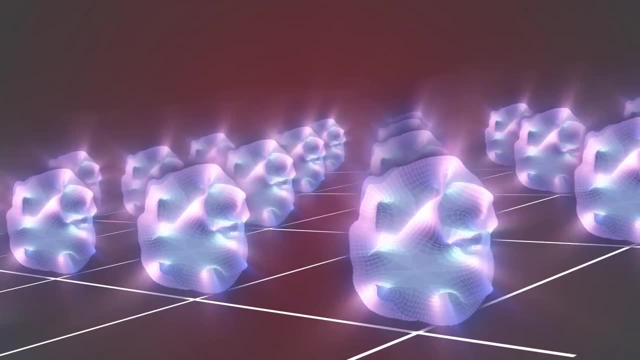 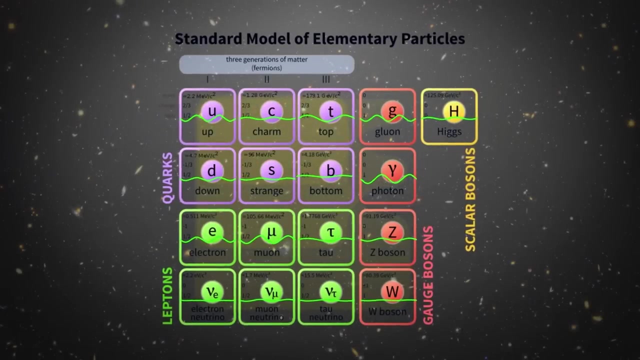 also corresponds to the number of particles. This is about as far as the similarities go. The multiple undetectable dimensions make string theory seem strange. The main idea that still drives interest in it is that it could result in a unified quantum theory by combining the standard. 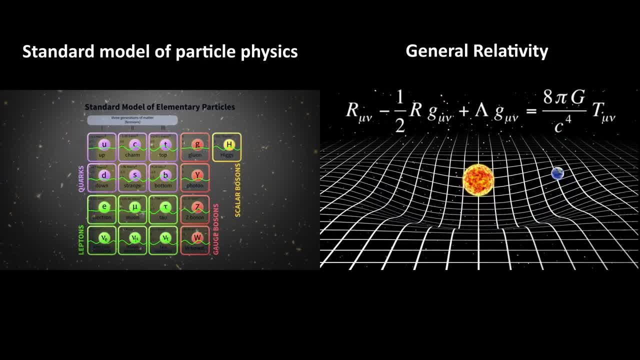 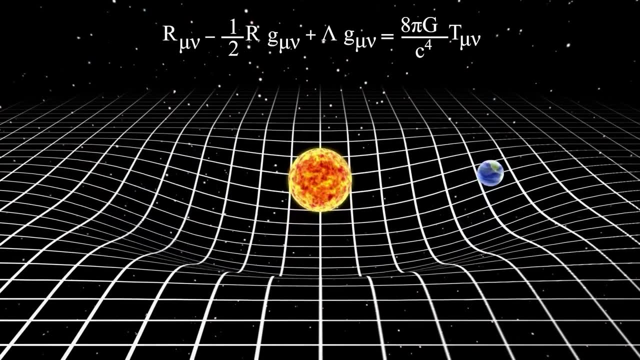 model which explains the strong, weak and electromagnetic force, with general relativity which explains gravity, And that's what we're going to talk about today. But general relativity is not a quantum theory and breaks down at the quantum level. It gives us. 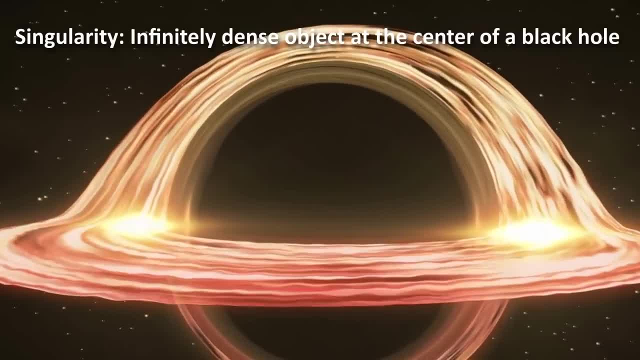 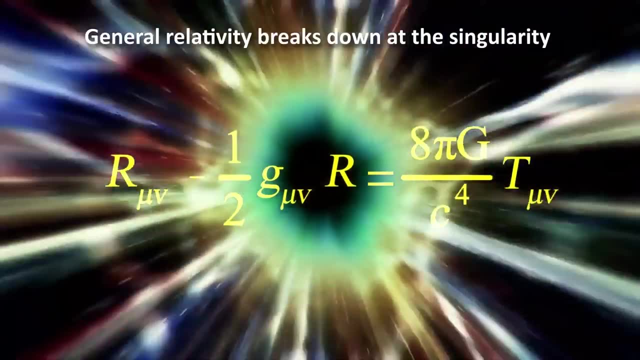 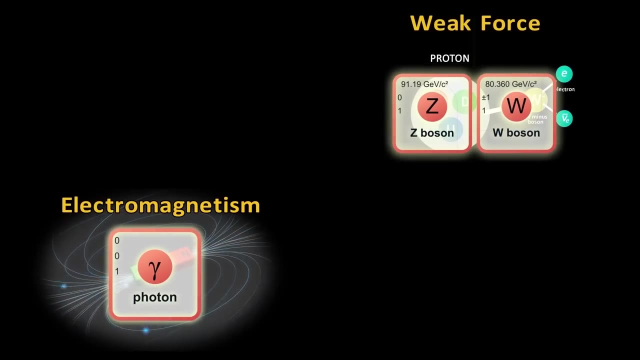 infinities. For example, it gives us a singularity which is an object of infinite mass density inside a black hole and at the big bang. This does not seem physical, so it's probably a glitch in the theory. Many physicists are convinced that gravity must also be quantum, because nature would not be. 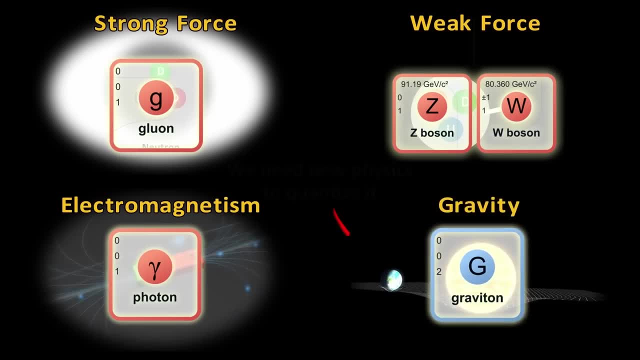 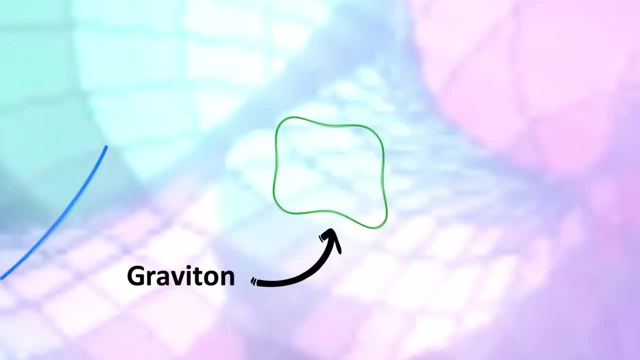 quantum for everything, but somehow make it so. So what does this mean? Well, we can't have a an exception for gravity, so we need new physics to quantize it. String theory, on the other hand, can be used to make a meaningful theory of gravity In. 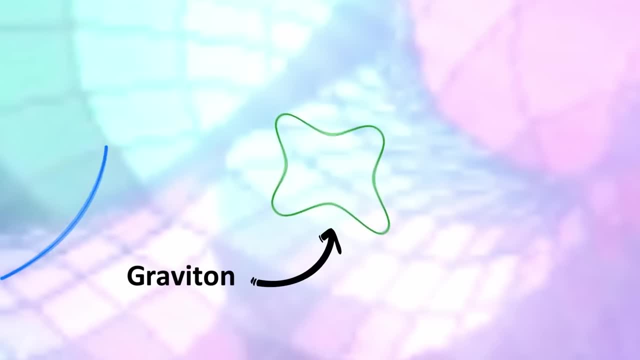 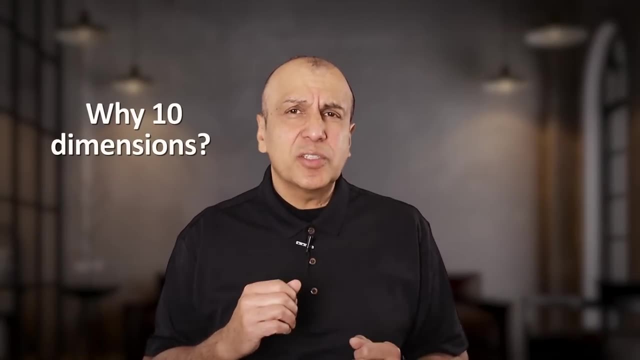 this case, the excitation or particle of gravity called a graviton is modeled as a closed vibrating string. You might be asking: why does the theory need all these dimensions? The simple answer is that its mathematics does not work in our four dimensions. It only works if we. 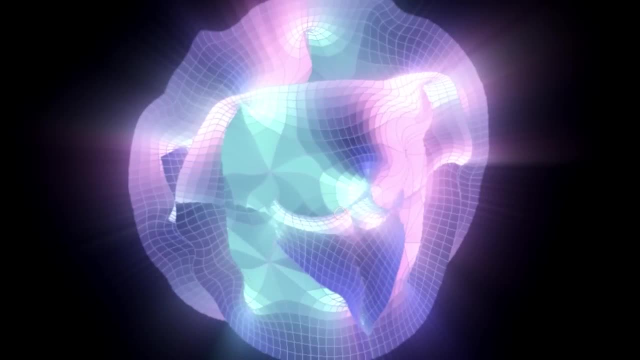 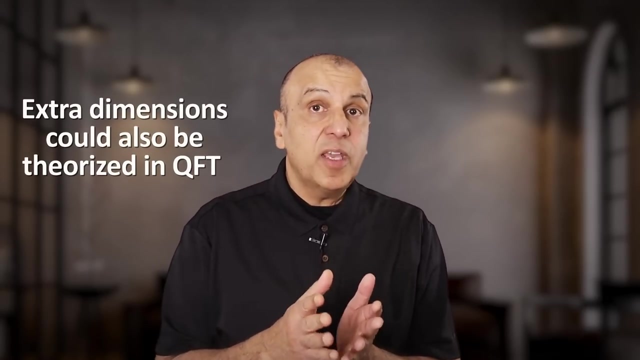 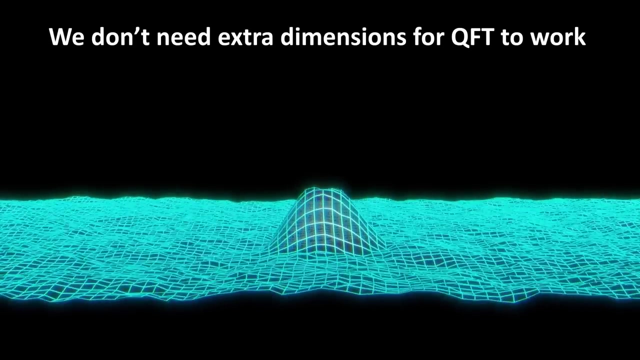 allow the strings to vibrate in at least six extra dimensions, or at least 10 total dimensions. Now I should mention that extra dimensions could also be theorized in quantum field theory, But so far we have not needed them to make the theory work. The math works fine in our 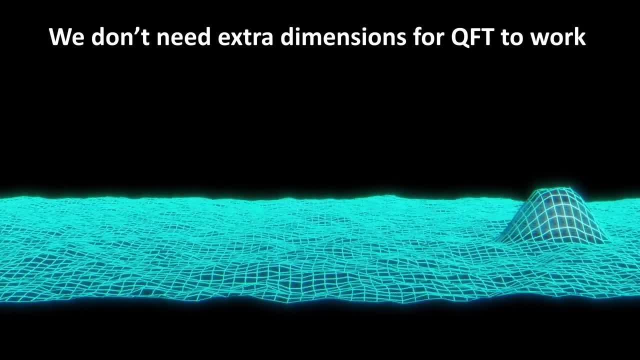 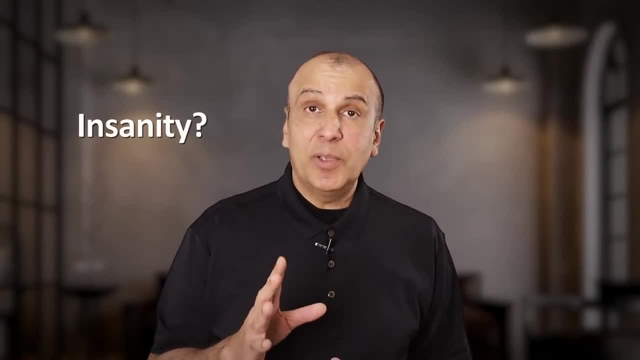 observable four dimensions as long as we ignore gravity. Now I you think that all this multi-dimensional talk is insanity. I wouldn't blame you. We're just there. We're just trying to solve a really hard problem, probably the hardest in all of physics. We can't afford to throw out any crazy sounding theory just based on intuition or incredulity. We should evaluate all crazy ideas based on their merit. Unfortunately, string theory doesn't appear to be a great alternative, because its predictions are either incorrect or untestable. 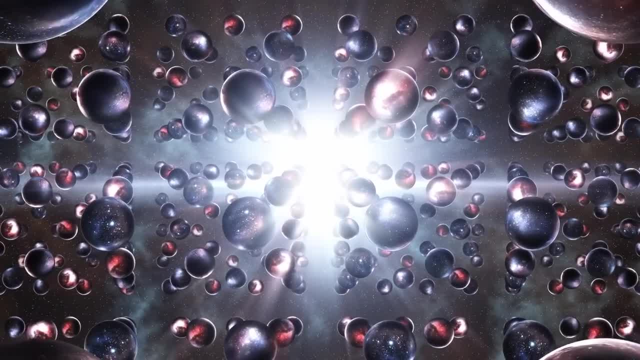 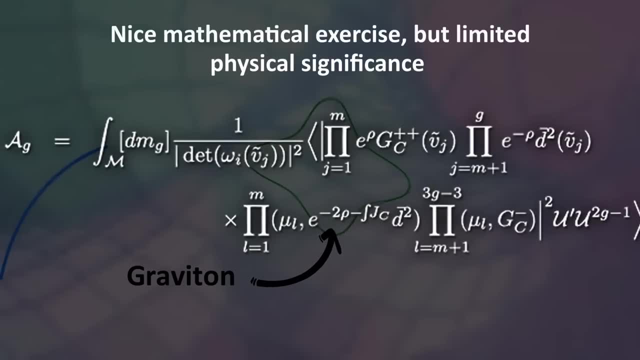 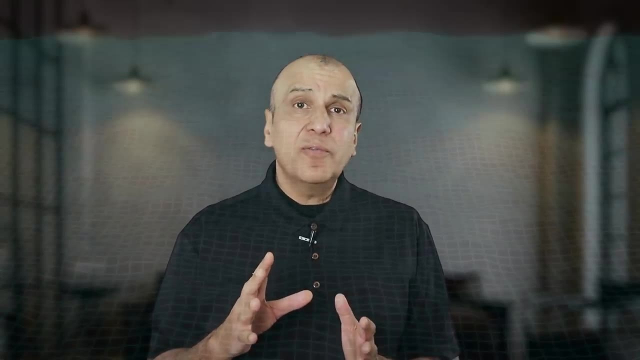 This is why it's getting out of favor by many physicists. On paper it nicely allows us to model gravity, but in practice it doesn't bring us any new answers. It's a good mathematical exercise but has limited physical significance. But keep in mind that science evolves and even though quantum field theory seems to, 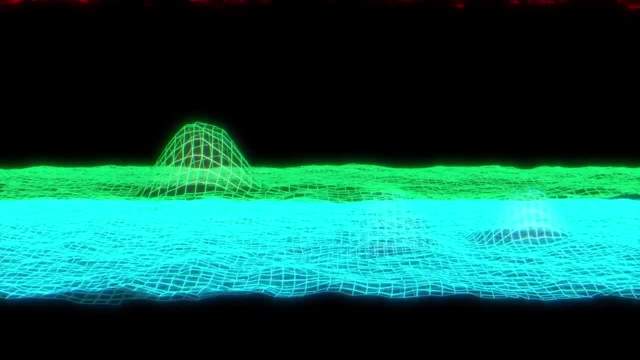 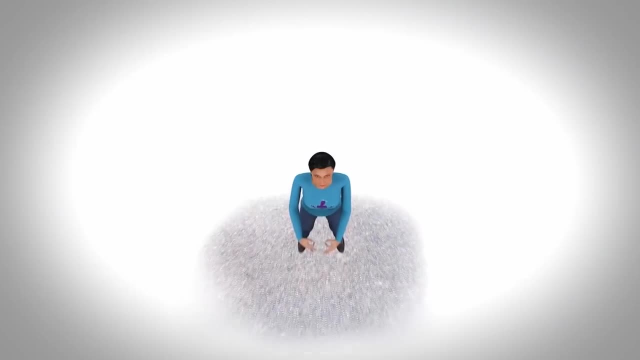 be the better framework today, it doesn't mean that it will remain this way in the future. We know that there is something beyond the standard model. We just don't know what that is. Could that be string theory? It doesn't appear so. 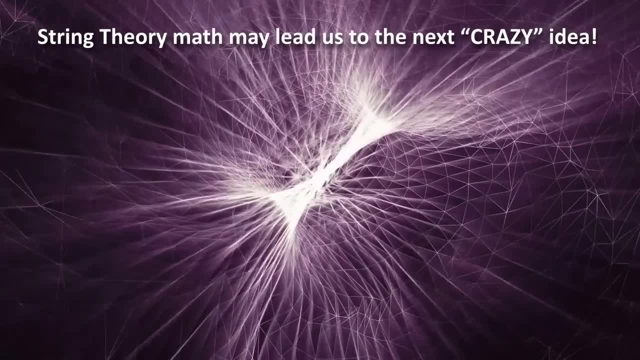 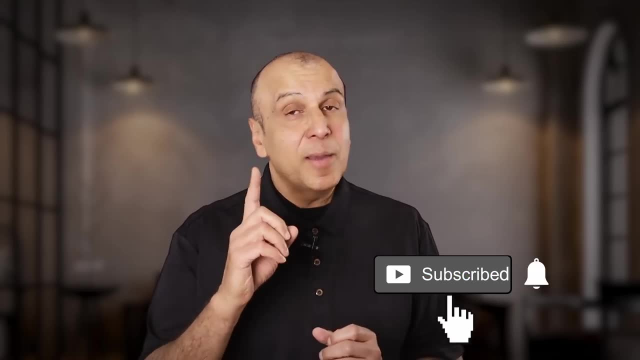 But its mathematics could provide the answer, The insight we need to come up with the next crazy idea. If you enjoyed this video, I think you might enjoy my video on quantum field theory and string theory That's coming up in about 5 seconds. 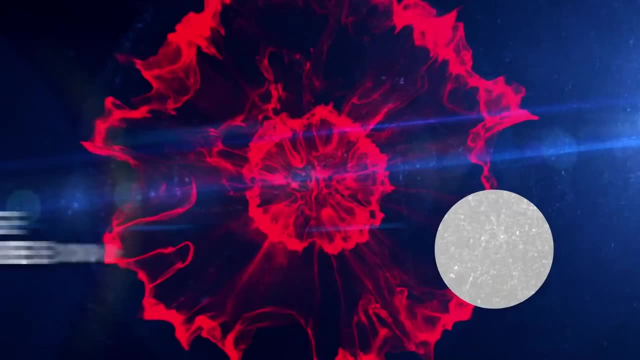 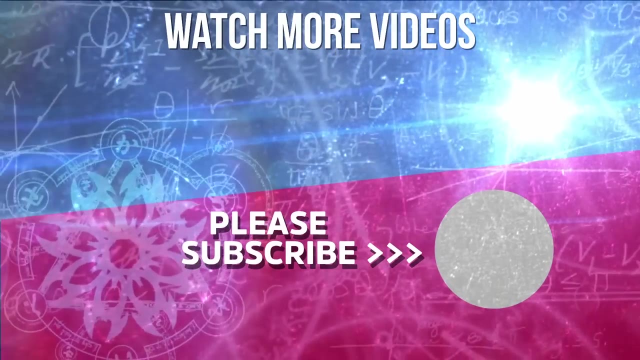 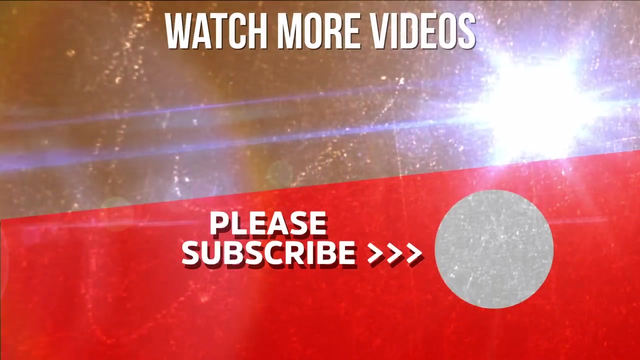 I'll see you in the next video, my friend Bye. 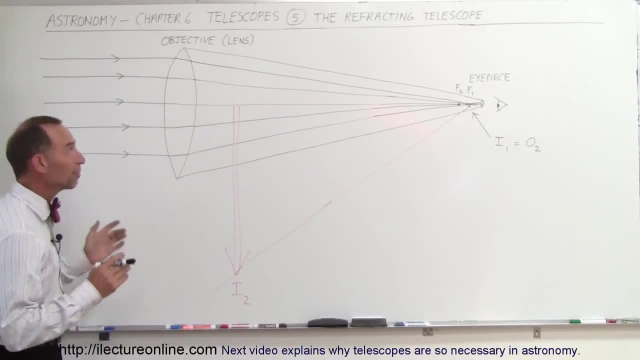 Welcome to Electro-Online. and now let's see how a telescope is actually built. We're talking about a refracting telescope, because there's a lot of different kinds of telescope, but the telescope that takes two converging lenses: a very big one up front and a small one in the back. they're both. 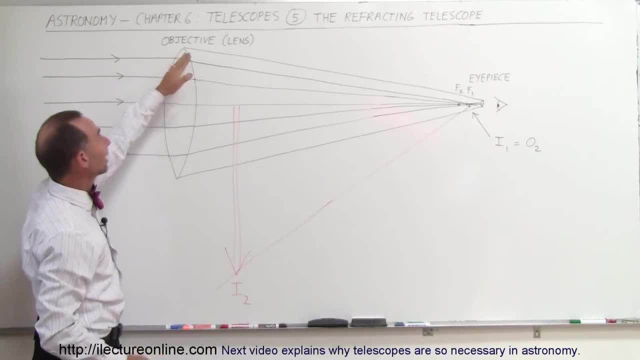 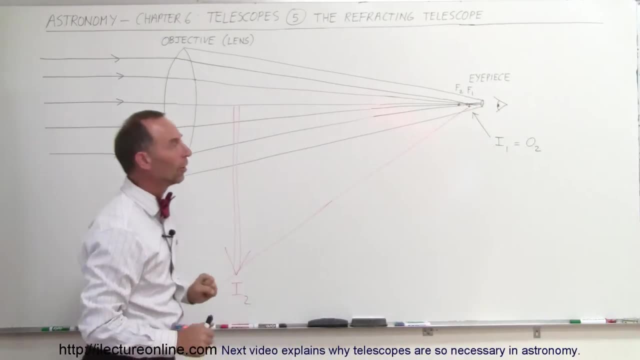 converging lenses, one called the objective lens, sometimes simply called the objective for short, and the small one in the back here the eyepiece to which the observer will look. So we take those two lenses and place them exactly the right distance apart, depending upon the focal length of these two lenses, and then you have yourself a telescope. 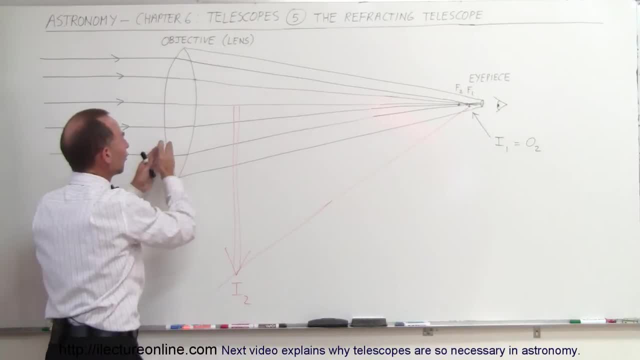 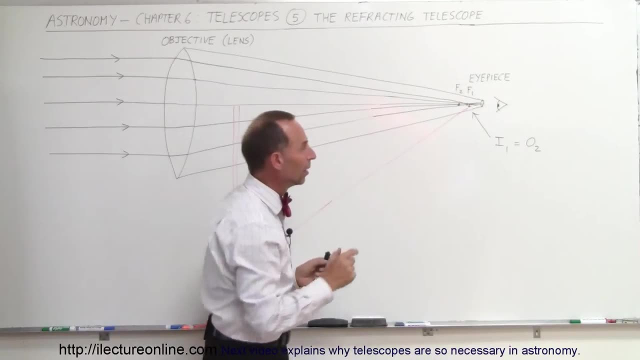 So the condition is that the first lens, the objective lens, has a very long focal length, and so you can see that the focal point almost reaches the second lens, but not quite. The focal length of the second lens is much smaller and, in order to make a telescope, you 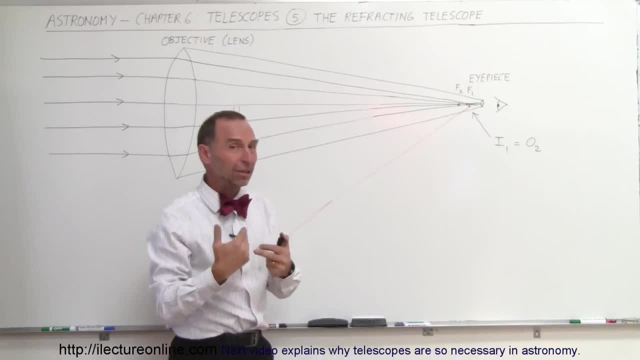 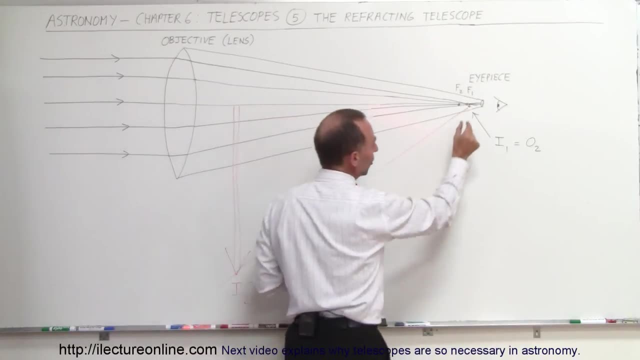 have to make sure that those two focal lengths overlap. if they don't overlap, it doesn't act as a telescope. So you want these two to overlap and then you have a telescope. There is usually a small amount of adjustment. you can move the small lens back and forth. 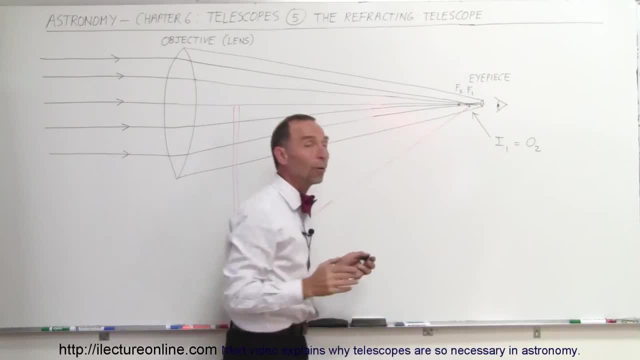 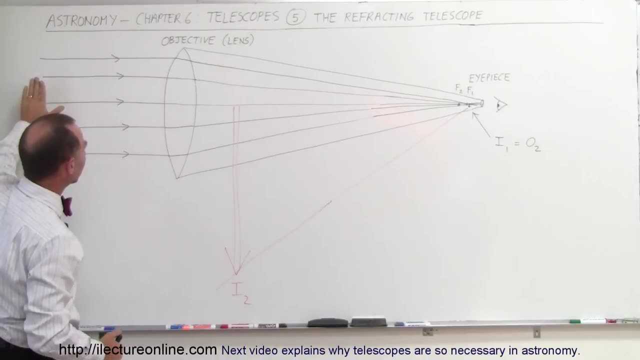 to make sure that it's focused correctly, to make sure that those two focal points are indeed overlap. So the rays come in from a very far away object, like a galaxy or a star. they come together? well, they don't come together. they come in parallel to the optical axis. go to the first. 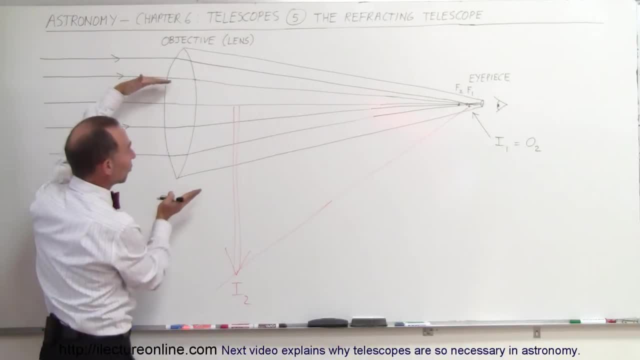 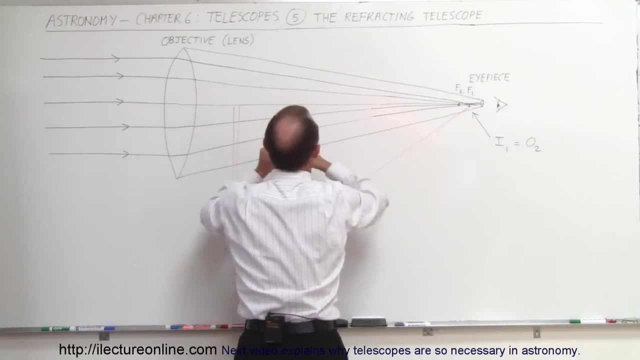 objective lens and, of course, since it's a converging lens, the rays will come together. the outside lines are, of course, the edge of the telescope. the inside lines are the rays of the light. so the light comes in, the light rays begin to converge and they finally converge to a point.